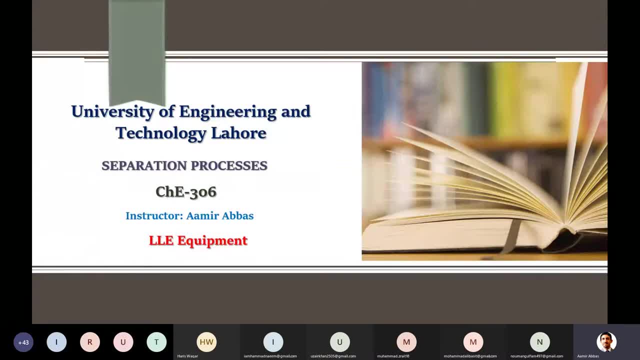 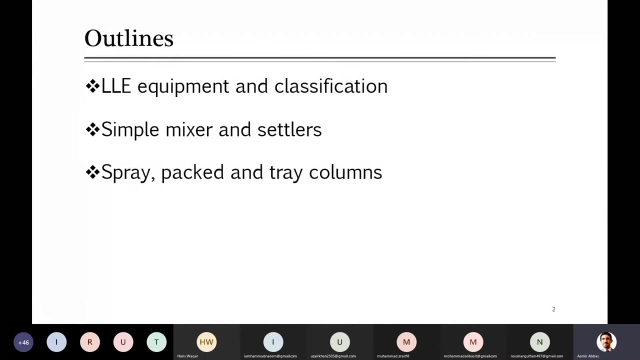 liquid extraction equipment. So quickly or briefly, we will go through the equipment detail which are used mostly for a separation involving liquid extraction And then, by next, we will start with the design of LLE equipment. So here we will just start with initially their classification and then after that. in this lecture a major discussion is related to 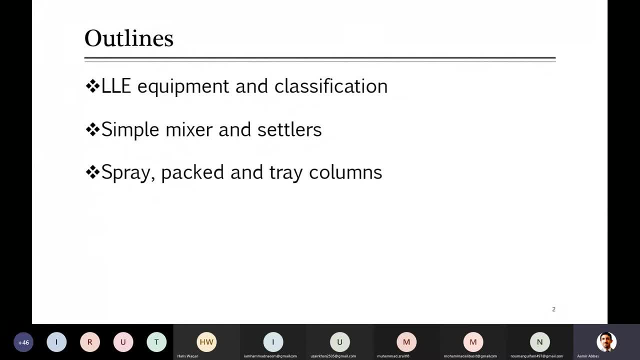 simple mixer, settler and then spray effect and tray columns used for LLE application. Although you know, these things already related to like either distillation or absorption, So same equipment can be used for both distillation and absorption. So we will start with the design of LLE equipment. 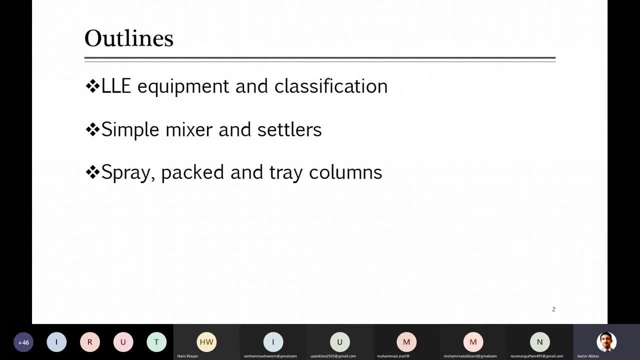 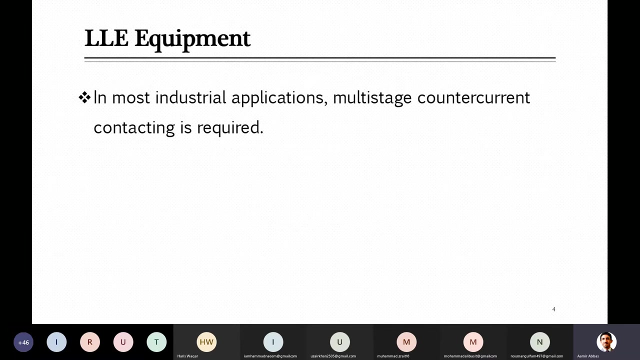 So, as yesterday was also, this point was discussed- that in liquid extraction for industrial application maybe you will need multi-stage counter contact. Why multi-stage was needed? if you remember, we discussed that when you will be bringing your feed as well the solvent in contact, There will be like not hundred percent transfer of solute from feed to the liquid usually. 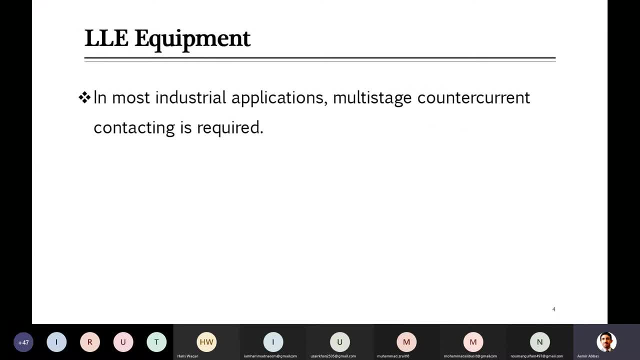 in one like stage, Then there will be still something left over in the feed. due to this reason, if you need more purity, you have to go for next stage, after settling, and so on. So, depending on the purity needed, you can need more contact between the solvent as well as the feed. 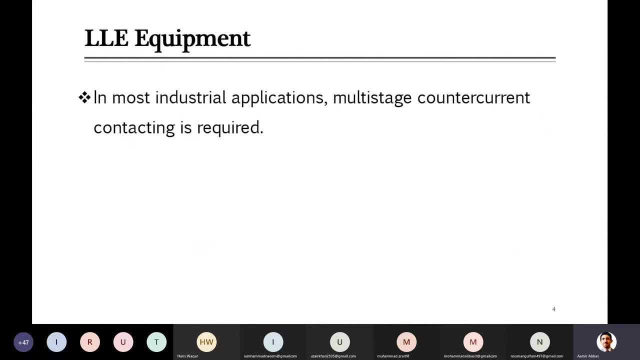 To remove as maximum as possible the solute from feed. So in those system which we have talked about yesterday, I told you that in liquid extraction equipment normally you will have something mixing equipment in which the contact between the solvent and feed is made. So after that, then you need. 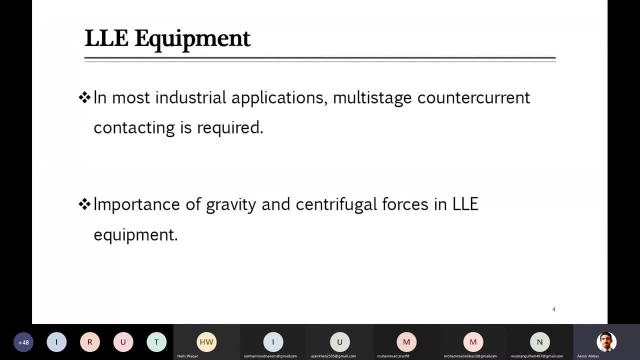 something called settler in which the settling, all the solute, is made. So after that, then, you need something called settler in which the settling, all the solute is made To removeברים or separation of two phases which were named as extract. 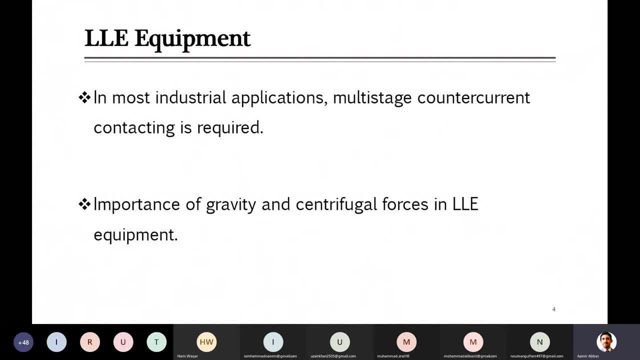 and raffinate takes place. so extract was the phase which is rich in the solvent and raffinate is the phase which is actually consists of the feed component. And in order to separate them, while we were discussing even the selection of solvent, there was a point related to difference in the density, so that two phases can be easily separated. 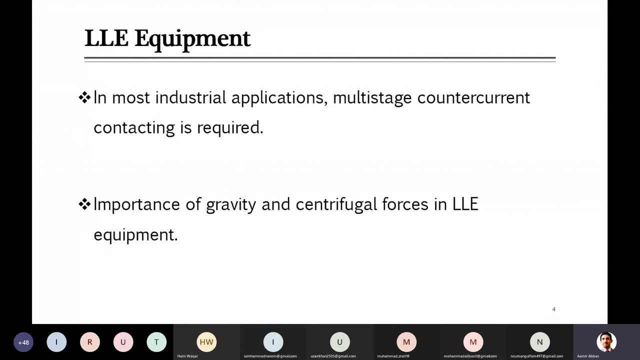 based on the additives and discover Colin c popularity where this percentage is easily and with high efficiency. so criticalbabíss much flexibility. the solvents, gravity, when we give time in a settling equipment. so due to this reason, gravity is important in liquid extraction equipment as well. another technique which you can use is the centrifugal. 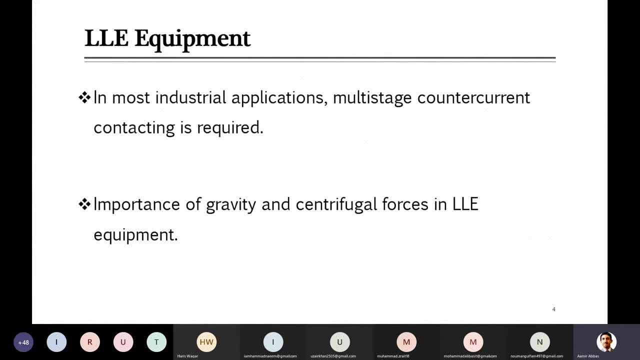 forces. you know, when we put anything in the centrifuge, uh that rotates, uh that, uh, that can be like anything in the form of a mixture, of a liquid, or maybe sometime the gas is containing the particle or anything. when you put it under the action of centrifugal force, then it separates. 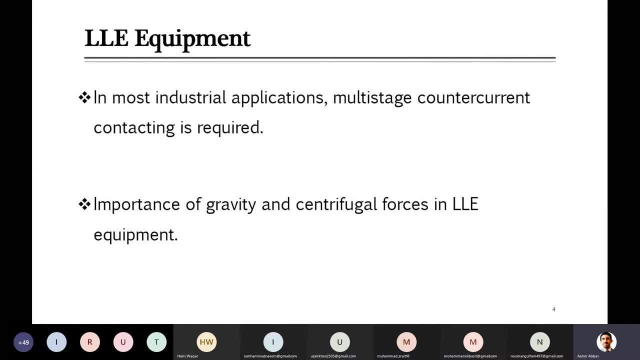 various phases based on the force being applied on uh different components inside the mixture. so in centrifuge, when it applies the centrifugal force, the phases are separated. but uh, that will be definitely fast as compared to the gravity action, but in this case, uh, in the centrifuge. 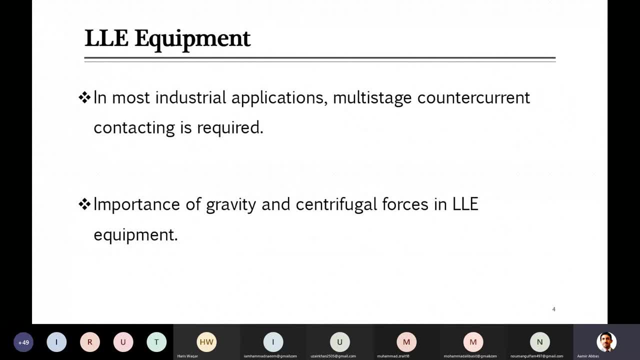 we need some force like uh uh force we have to apply with the help of some external energy source. you have to install some motor which, like, provides that rotation. so, due to this gravity, is this preferred, in case you have a sufficient time and can go with that? uh, most of the equipments uh here in like which are used. 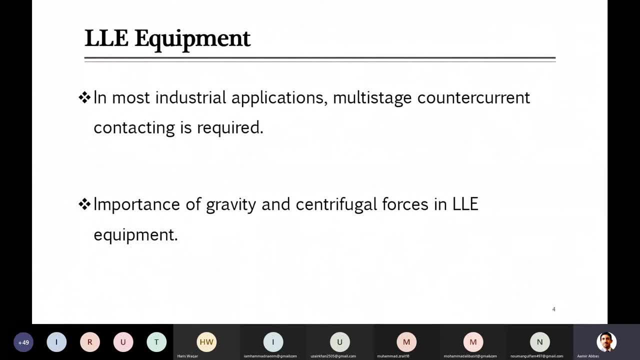 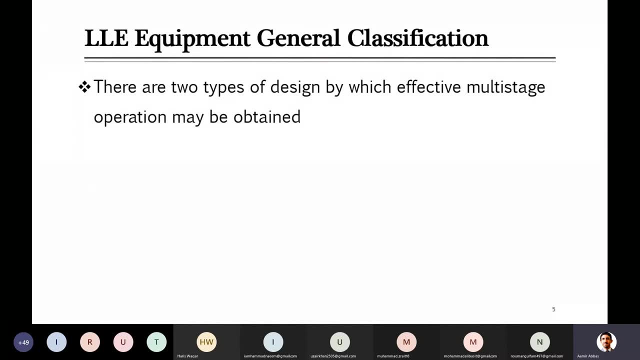 parallelly and if you are using mix link and then settling tanks, they work on the gravity principle. so when you look at the design of uh equipments used for lle, so uh, effective multi-staging operation, as we are saying that we will need more than one stage to go for the complete separation or removal of any sedu from. 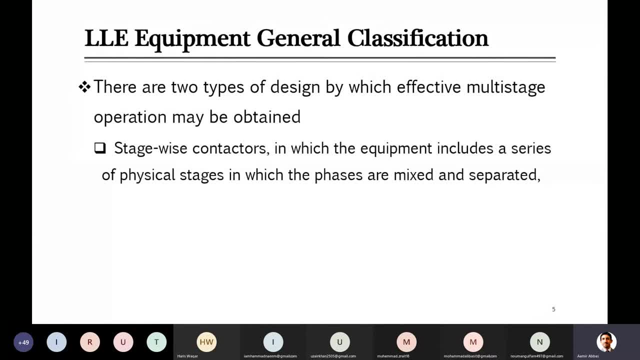 feed. so, uh, they are. just there are two types of interaction or design. if you can observe, uh, they are named as, like state state wise conductor and those are the one which we have already talked about. are, you know, somehow lost and just discussed, uh, the things which i have just discussed? so, 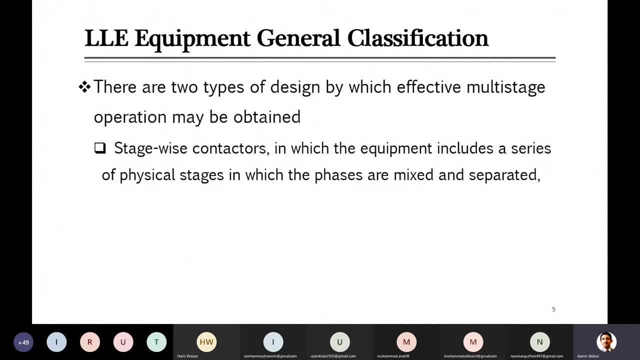 in those there will be equipment, uh, in which mixing takes place, and then there is another equipment in which separation takes place. due to this reason, we are calling them stage wise conductives. there is one like vessel in which feed and solvent are mixed, then there is another. 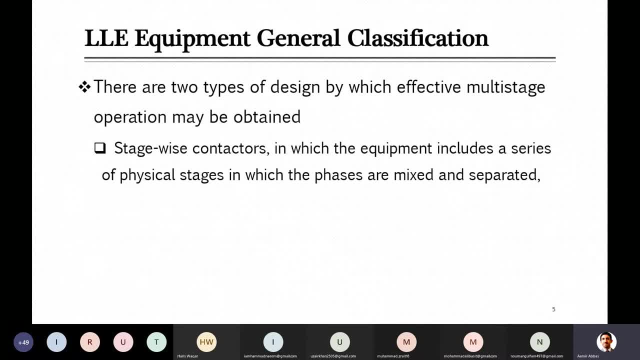 vessel with in which you give them time to get them separated into the like two separate phases and then, when they are separated further, raffinate is contacted with the more solvent to extract more solute from the feed, and so on, while the other equipment- they are generally named as differential- 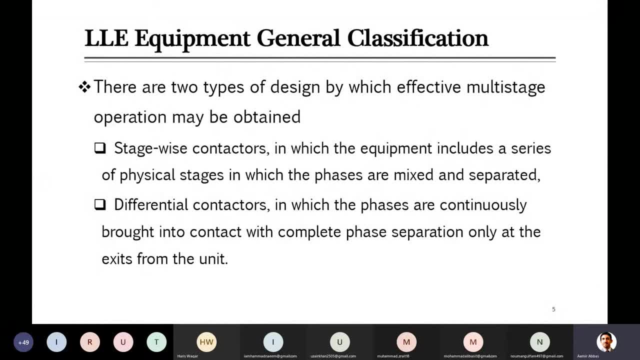 contactors. so in the- in those i mean equipments- usually phases are continuously brought in contact throughout the equipment. these equipment definitely will be large in size and in the same equipment when the phases are leaving, they, like these, are large size equipment. and later when we discuss, for example, if you have tray based cover, so inside tray tower, there will be a number of. 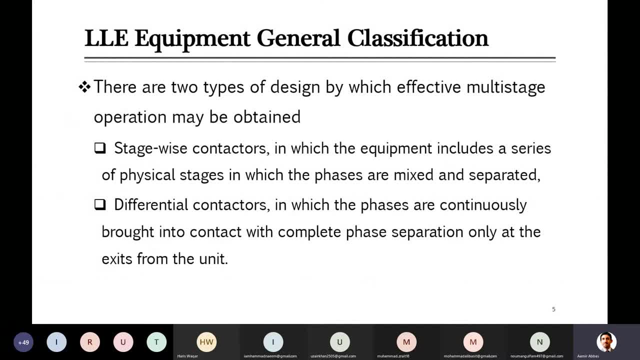 stages, number of trays. so when two- liquid solvent as well feed, will be coming in contact and then at the end of the day, uh from the same equipment heavier feed will be leaving. uh like heavier any of those, either that is the feed or solvent that will be leaving from the 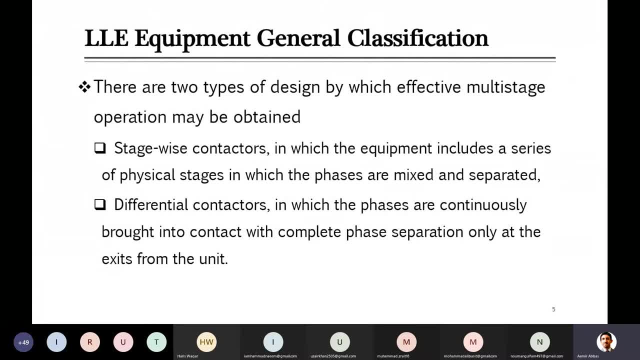 bottom. that is a like either raffinate or extract, and the lighter one will be leaving from the top. so in the same equipment, like both, contact as well as separation of the phases occurs, uh, but definitely in these equipments they should be of sufficiently large size so that 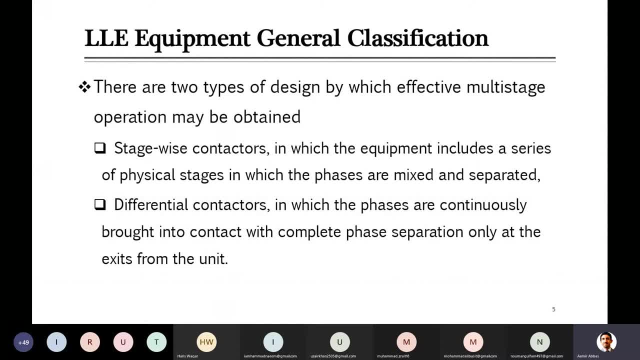 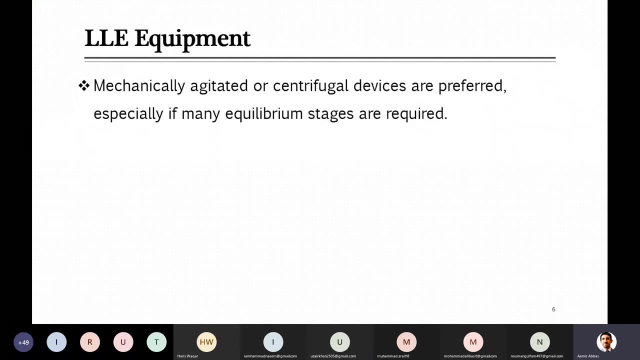 contact as well as then settling or separation of the phases can take place, but in the other you need separate, uh, like a system for separate contact as well as for separation so that that can be like small sizes. as you know that already this mechanical, agitated or centrifugal devices they are preferred for. 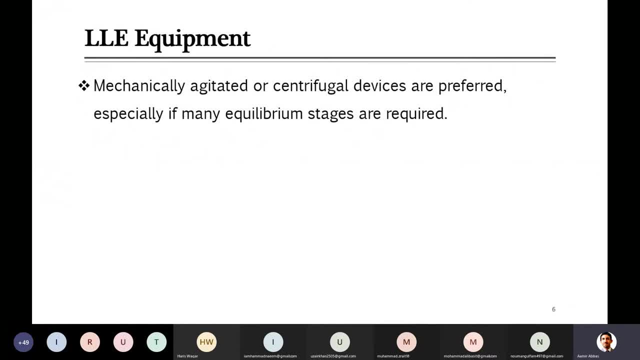 especially when you need many equilibrium stages. the reason is like when we are bringing the liquid, sorry feed and solvent in contact. so if we can educate mechanically, that will help you to like better mixing in that because, as i said, that in those kind of equipment which consists of like, 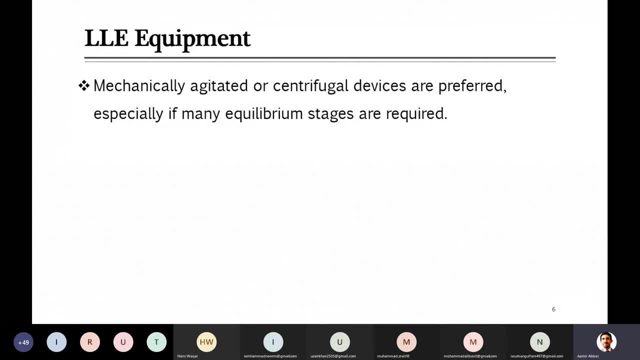 mixer set, the mixer settler. so in those cases mostly equipment are small size, so you need some extra force to increase the contact between the solvent and feed. and then later- uh mean like in centrifugal devices, are uh gravity. gravity is natural, but if you apply centrifugal force, that 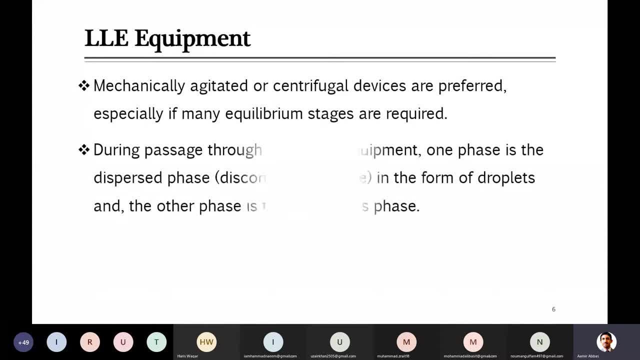 will help you to like quickly, quickly settle or separate two phases uh. so whenever uh feed as well as the solvent are passing through any of the equipment, extraction equipment, so uh majority when you bring them in contact with each other. one phase is like dispute space, discontinuous phase, how we have to disperse like that is uh, that can be either feed. 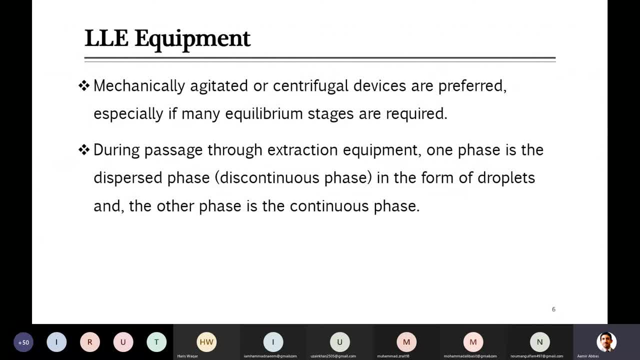 or the solvent and that is introduced in the form of droplets, like you pass them through, either spray such kind of devices so that it can be just, uh, dispersed. it can be broken down into the small droplets as compared to the continuous form, while one one other phase will be like continuous. so 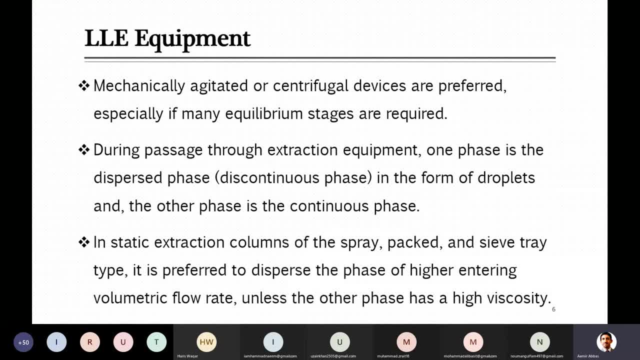 when they come in contact, the mass transfer will increase in this case. so in static extraction column, uh, static extraction column like, uh, there you are not introducing something like agitation, or uh, mechanically, uh, like you are not disturbing inside the equipment. so in those type of equipment like spray packed or sea tray type, uh, so, uh, in those kind of equipment usually. 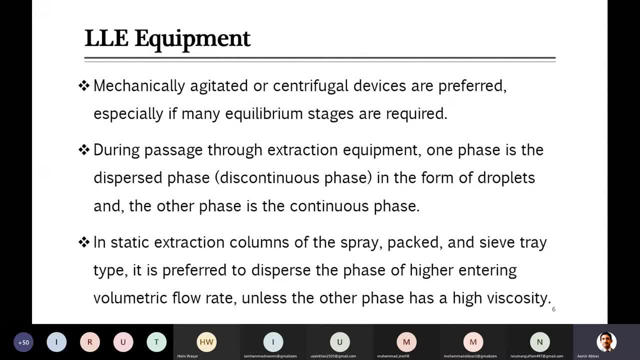 dispersion of higher entering flow rate feed is uh like done: or we disperse, or this continues the phase which has high flow rate. so uh, otherwise, the major criteria is to disperse that phase which is of high viscosity, because if it is of high viscosity it's like. 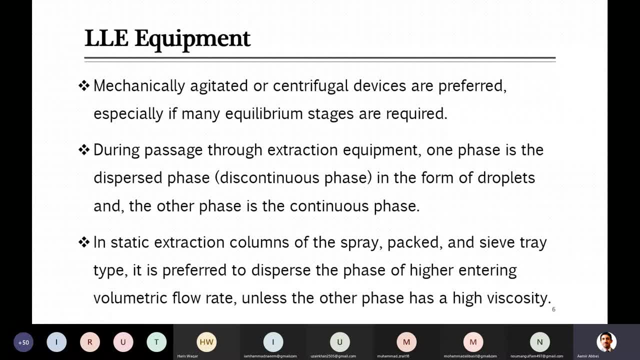 mixing with the other fluid will be less so. anything with the high viscosity is usually dispersed into the droplets so that it can make better or more contact with the other phase, while in other equipment where you have simple, already mechanical agitation, you are using some mixing elements. so in those kind of like equipment you don't 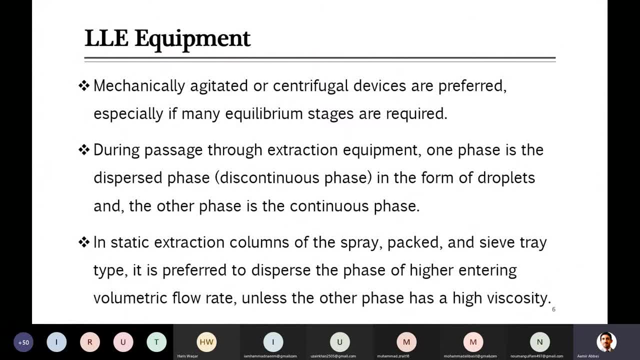 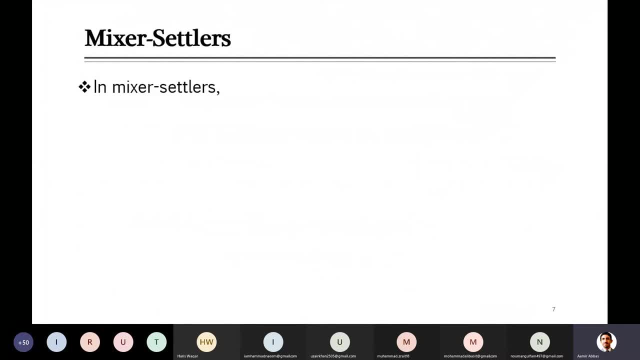 need a separate like distribution of any phase in the form of droplets. so first, equipment which is used for this purpose is named as simple mixer settler, and these are the simplest devices uh which are used for liquid, liquid extraction. uh, in that uh, there will be as 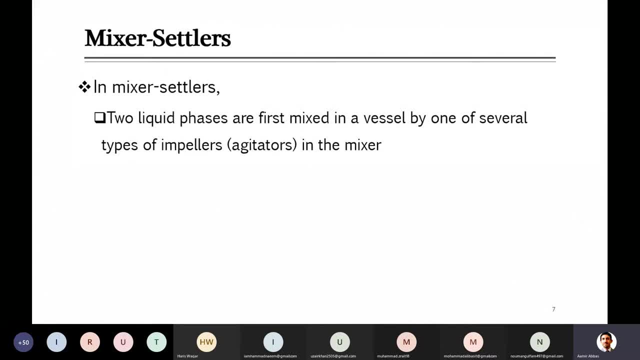 again clear from its name that there will be a mixer and then there is a settler like this: uh, i suppose we have one state, so in that one stage there will be one mixer, one settler. suppose it is two stage equipment, then there will be like two mixer stages and two, uh, settling stages. so here two liquid phases, which 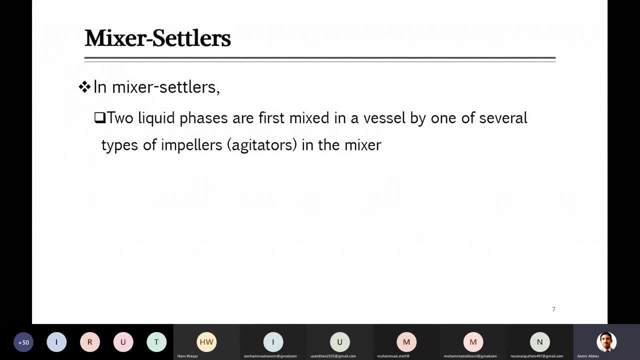 are feel and solvent. they are first mixed in a version uh so by one of the several type of em PUBG'th we will look in next slide. uh, there can be a different type of em- piping, Stromae, Reman, catgrass material- so they are used for the mixing and then you give them a time to get separated in the additional stage on the latter, where they will operate uh as well by next. 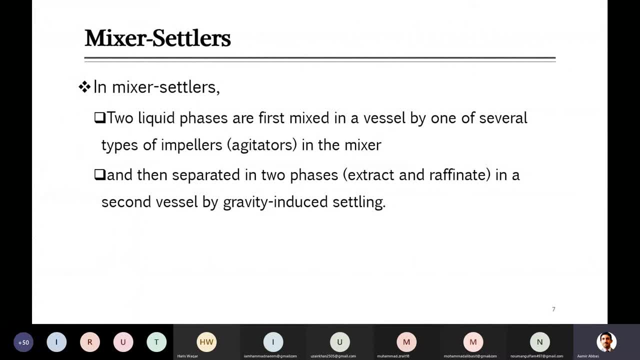 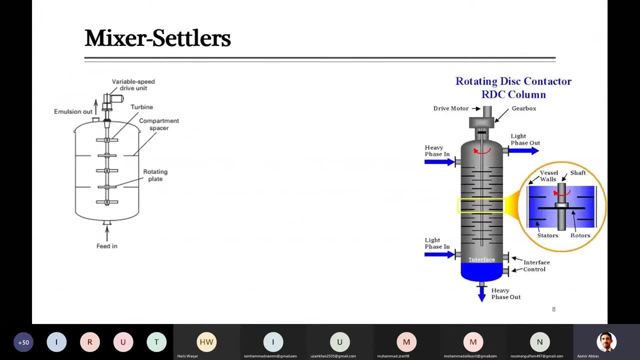 into a strict and ratcheted phase in a settling vessel. that can take place majorly in these equipments. that takes place by gravity. so here are, like equipment, first stage, that is the mixing stage, in which you can see that we introduced feed as well the solvent, into the equipment. 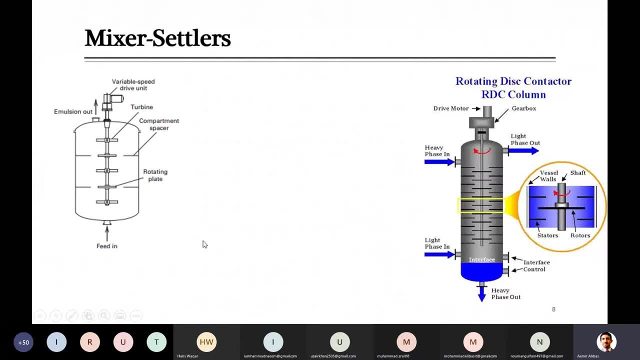 one diagram shows on the left side, in which, as he said, feed in. so actually both feed as well as, like the solvent, they are introduced together from the bottom of the equipment and inside this then there is mixing. you are applying something, some mixing element, in which mixer are located. 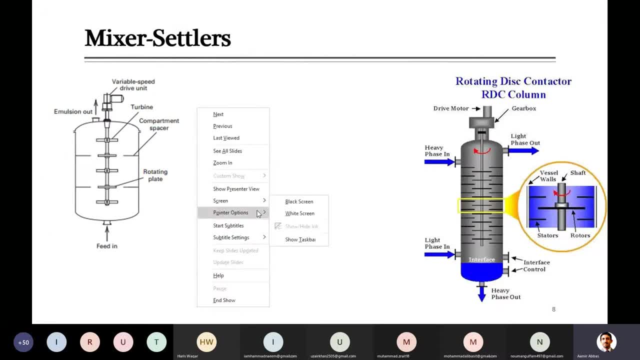 and then you can use it like for for mixing of feed with the solvent to increase their contact. when we are mixing there will be definitely breakdown between the continuous phase. they will be dispersed here when they will come in contact with these impeller elements are rotating plate so they will be definitely dispersed and will make more contact. 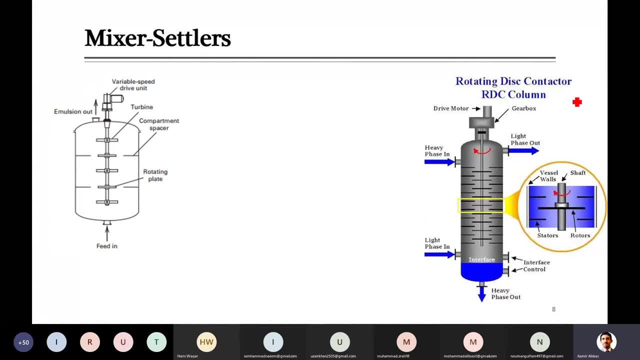 while in the other equipment, like here, we call it rotating this contactor. this is the same type of equipment, but here what we are doing? this, oh no, this is not related to this, because in this kind of thing, but actually this is a wellsprings network ofure. so investigation is of where the 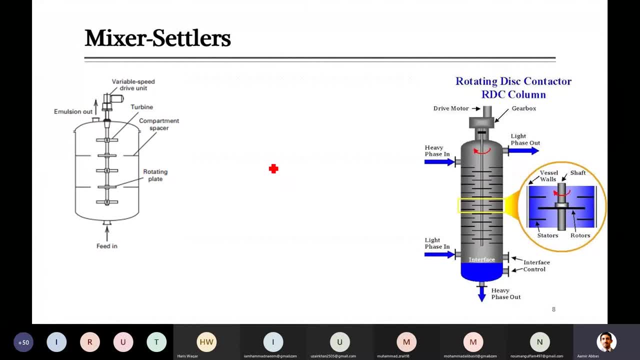 liquid would across from the solid of the solvent is flowing, it will fold upwards. and here you see that on this occasion, we actually are involved in this processes and we are using, like the conveyor, oportunity and the air flow, and so on. um. there are two mechanisms, one of which 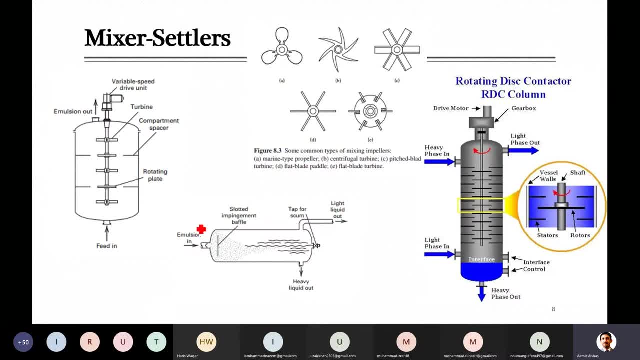 we are see that you can see here. here is våask lim, a piece of an object. this is the electronic vertical orbitalATION and this is data signal 3D. you can see that there are the based techniques, the takes place and, like those phases which were mixed inside the mixer, they get settled down. 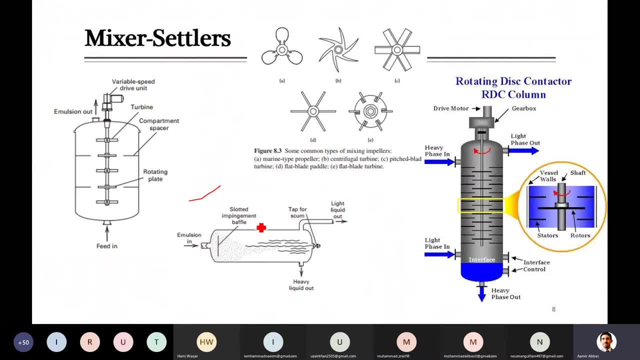 inside the next vessel, and this kind of vessel can be either horizontal or vertical, in which emulsion, as we said, like coming out from this mixing equipment that will be entered inside this and when you give them time, they get settled by gravity heavy from the bottom and 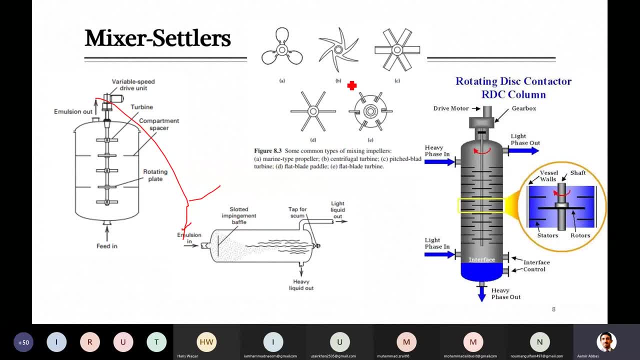 lighter from the top. so there can be different type of, like this, rotating elements. they can be used inside the various equipment to increase the contact between these two phases. so here different type of- i mean different types- are mentioned, just for your information that impeller of these various kinds can be used inside these equipments. 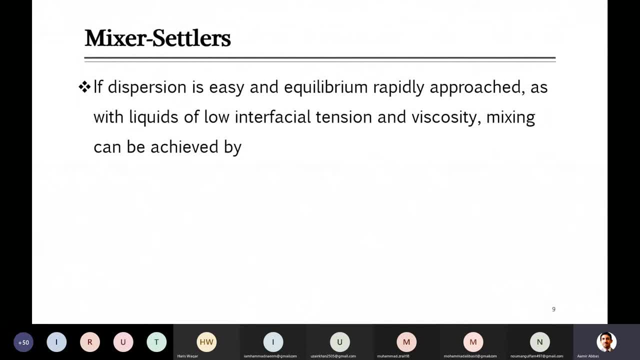 so in in in these kind of equipment, which are the simplest equipment in which mixing and then settling is taking place. so, uh, if simple, let's say dispersion, is easy. dispersion, the contact between the two liquids, and i mean the achievement of their equilibrium, if that is easy and that will. 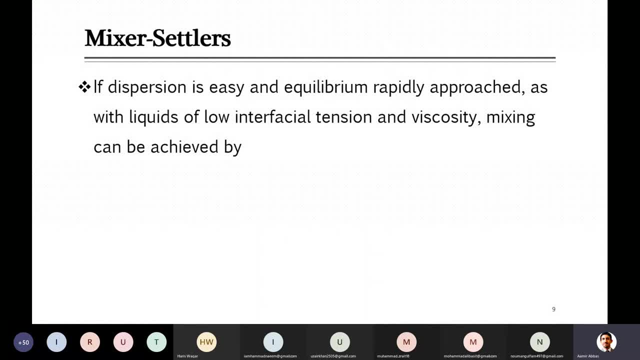 be easy in case of like, when both of the solvent they have low interfacial tension as well as the viscosity. uh. so in those cases, so in these kind of equipment, which are the simplest equipment in which mixing and then settling is given instead of flexings, when you you have additional extra items there, you can set them. 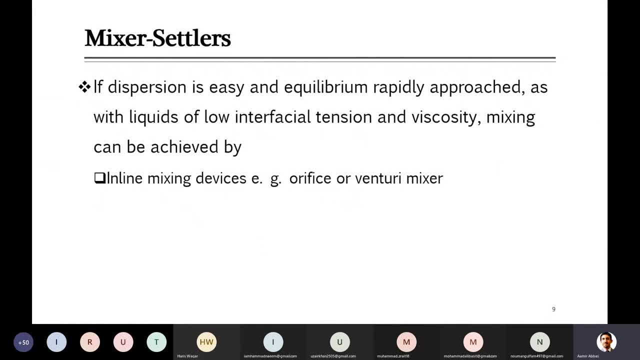 to give it more tension to. then we have the aqui's three place or First Patient voucher automatic for those products. that's okay. so when you, when you have a forcing method, for example you put your theř Petrol or what seraman man, for example, you know that when we use these oil test or venturi plates or 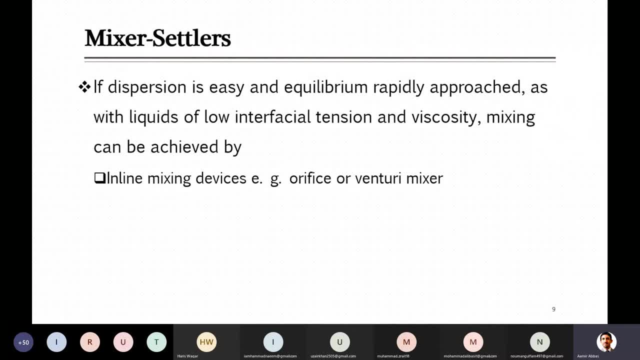 there, uh, some disturbance takes place for the fluid flow and there can be no mixing can take place inside the line. even so, what you can do is to introduce feed as well as solvent that can go out and convert for the 내가. it is to replace it. one let it. so. now i will let you know how to start. toножar ke transc. ***which is a very 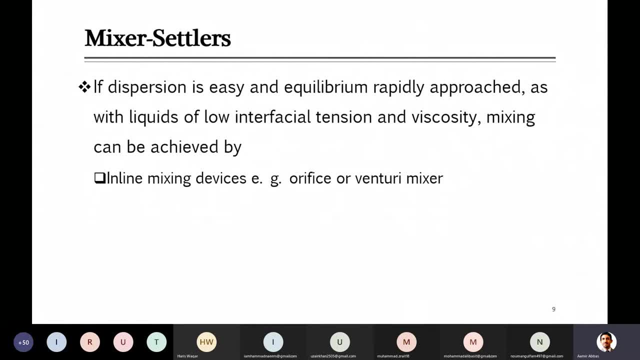 in a line and just install these orifice or venturi mixer, so their mixing will take place, although that will be not that sufficient as you do in a one large vessel, but here they can be easily mixed with each other. small scale application: you can even use this or the other cases for 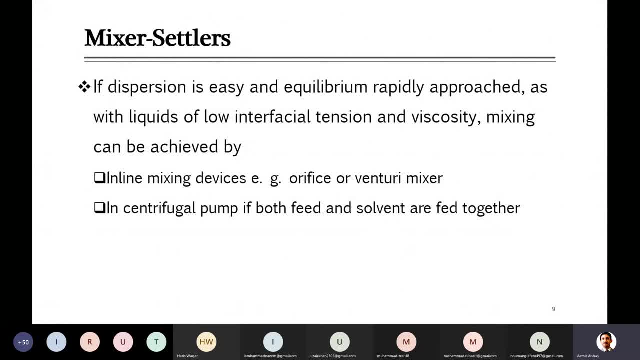 example, you know that inside the centrifugal pump when we are pumping the different liquid, so they can be like introduced at the inlet of this main pump together and when they just pass through the impeller inside the main pump they can get mixed with each other and that master can take place. or 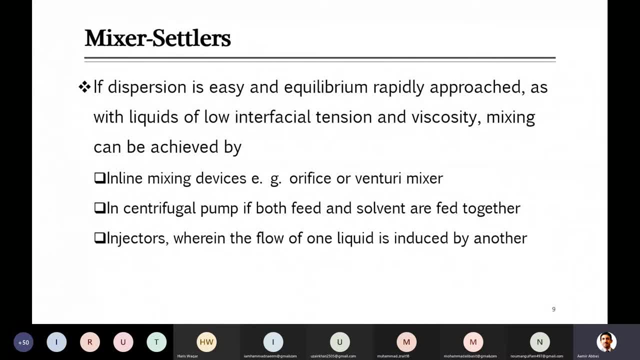 in other cases simple. they something called injectors, so like we have flow of one liquid introduced by another. injectors are such kind of devices in which one fluid is flowing to this, reduce the area or something like that, So like venturi- and another liquid. when comes at that point, actually vacuum is created and that 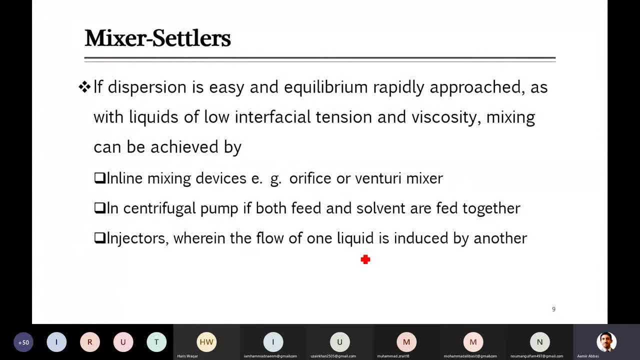 attracts the other liquid to its inside. so that will be like that equipment. that is the simplest arrangement that can also be used, but in major industrial applications definitely you can't go with these small mixing devices or these inline mixing devices, so you will need separate vessel in which mixing takes place, and that's the reason why we are using this orifice orifice. 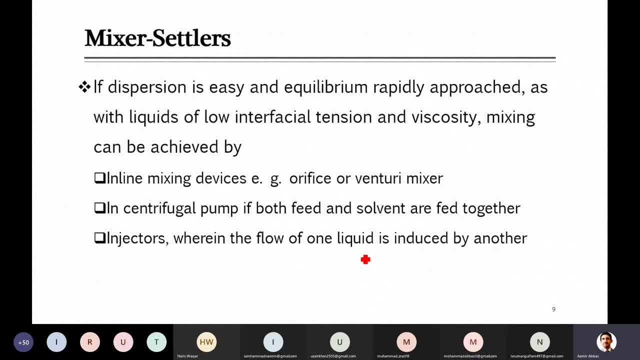 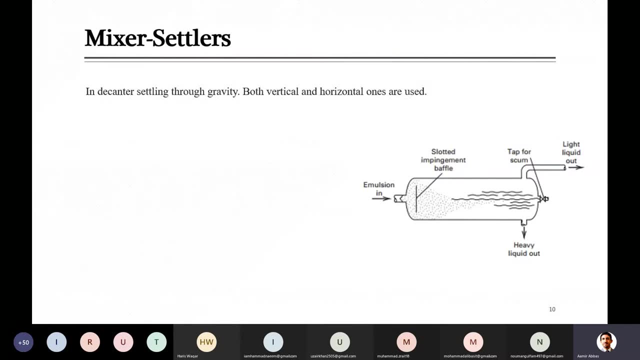 Then you get them settled. definitely if this mass transfer or this separation can be achieved in these small inline equipment, so they could be helpful. but on large scale definitely it will not be that efficient. so in these kind of equipment the settler are- we also called it like decanter. 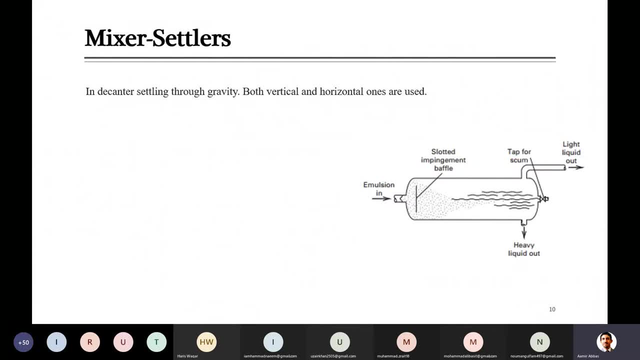 decanter is a dead device in which the separation between phases takes place due to the gravity. it also creates some various building. so decanter is that device. so in decanter, here setting through gravity like it is simple vessel in which you settle the different phases through. 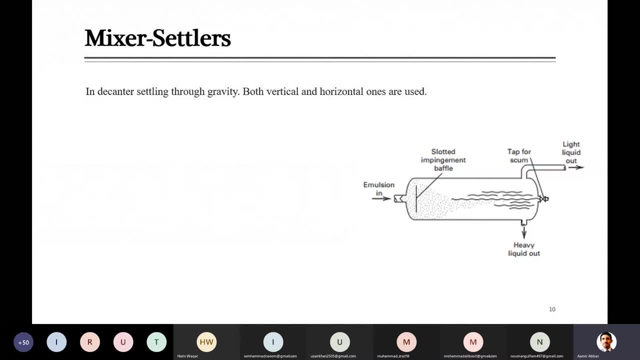 gravity, so they can be both, as I already mentioned, vertical as well as horizontal. so you give them some time. integrated certain, these are definitely large size vessels and in which fluids are introduced from one side- they are coming from the mixing unit- then they will just pass through. 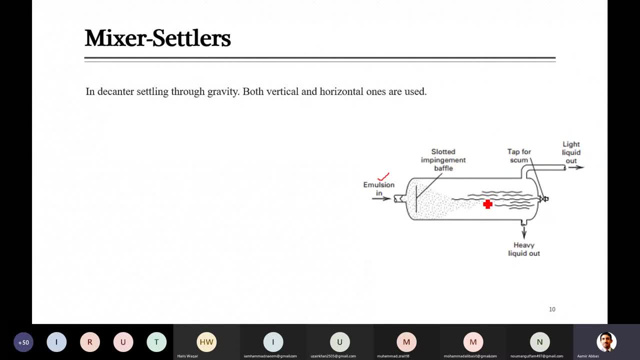 this while moving. they will just get separated based on the gravity. so here in these equipment, there is installation of impingement baffle, like baffles- you know- I think you are studying heat transfer and you are aware about the baffle. so here the purpose of this impingement baffle is. 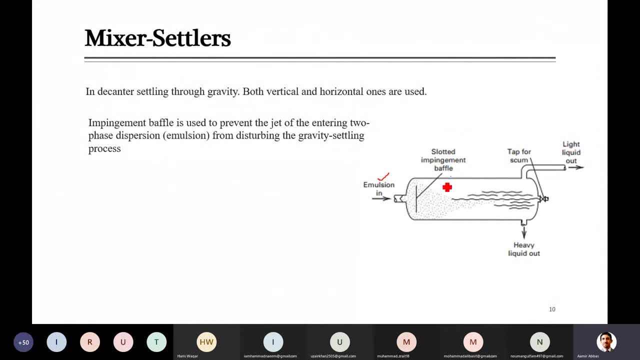 just to avoid the destruction of two phases which are already separated, for example. if we don't install this any, anything which we are not going to install, then we are not going to be able to do so. this is the purpose of this impingement baffle. so in these equipment there is one major problem. 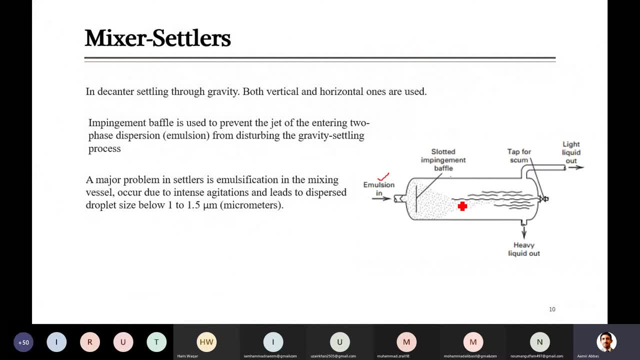 and that is related to a formation of strong emulsion. so hopefully you are aware about emulsion. emulsion is this dispersion of small droplets of one liquid into another, and those droplets are dispersed because those two solvents are actually not miscible with each other, or two liquids when they are not. 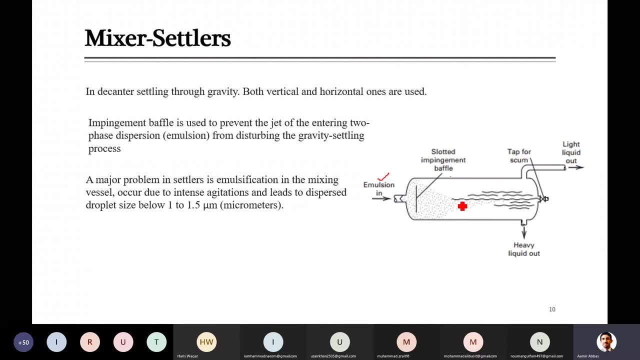 miscible with each other. you bring those two liquids in contact with each other and if you will mix them- although, as it is clear that they are not miscible, they can't be mixed together. so what will happen? one of those, which is the emulsion of the liquid, which is the emulsion of the liquid, 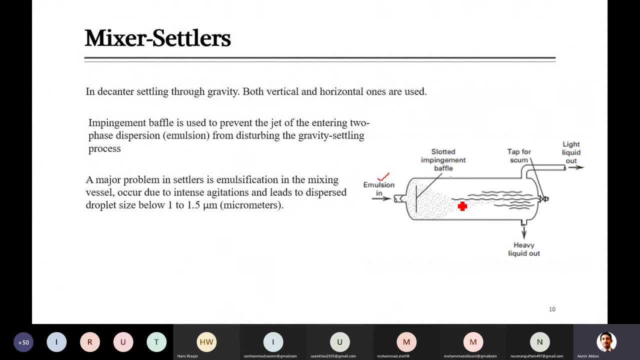 those which is usually in small amount as compared to other. that gets this dispersed inside the other liquid in the form of small droplets and those sometimes like, as we said that these are mixer and settler devices. so inside the mixing equipment, if you provide strong mixing and if 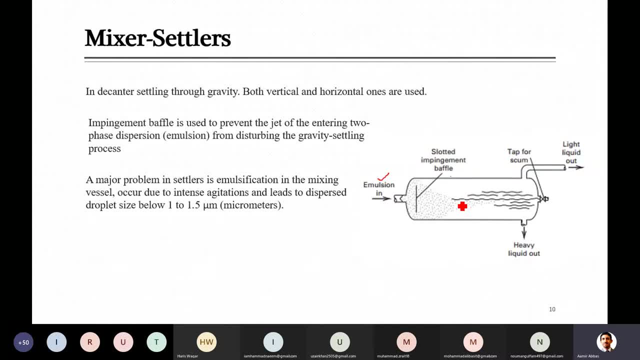 emulsion is formed so that immersion sometimes can become very strong. and that is mostly if you do one more therapy situation or the other is usually very familiar, this kind of situation fine, we would also track whether there cause of diferral causality that can occur in an example of this problem. so let'sysita here serious. and that were. 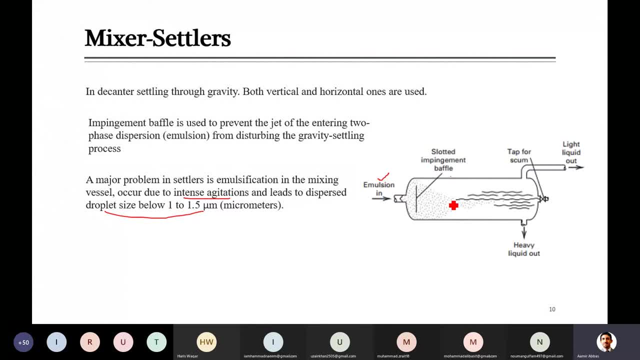 connect those small droplets with each other and get them settled. so, uh, due to this reason, then you will need some external force, and that external force, uh are treatment, for example, a demulsifying agent. maybe we have to add some other chemical which help those uh, i mean small. 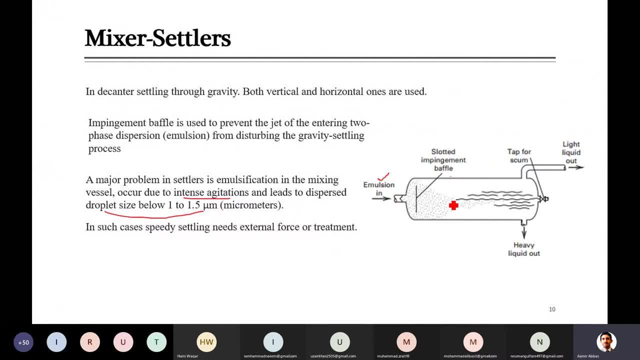 immersion for droplets to join together and form large droplets so that they can be settled in the form uh, with the help of gravity, either towards bottom or maybe, if they are lighter, they can go to the top. so, uh, this is one problem as well, the other problem in these kind of use of these: 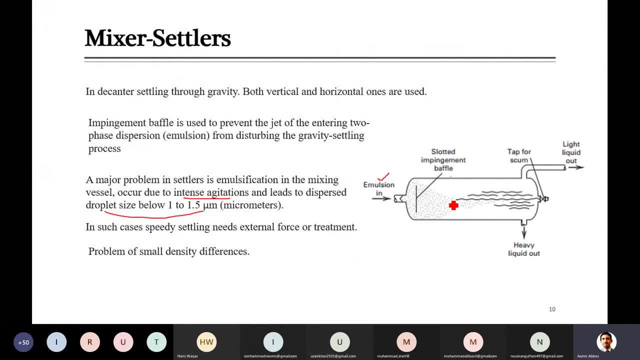 equipment is like density differences. density difference are small. definitely there will be not complete separation inside this settling device, although this density problem is like for all of the equipment. due to this, when you are going to select the solvent, you have to take care of this uh point, uh like, so that you can easily get them separated. 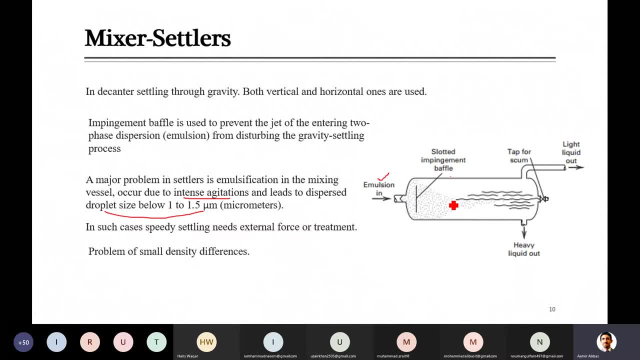 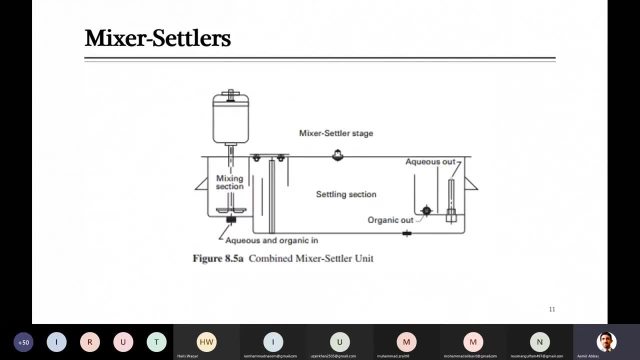 later when, whenever you want to separate, either inside the same equipment or inside the separate equipment like a second. so here in this diagram from your textbook, like, we have a mixer, settler devices and they are combined, although here again mixing is taking place in a separate part, like 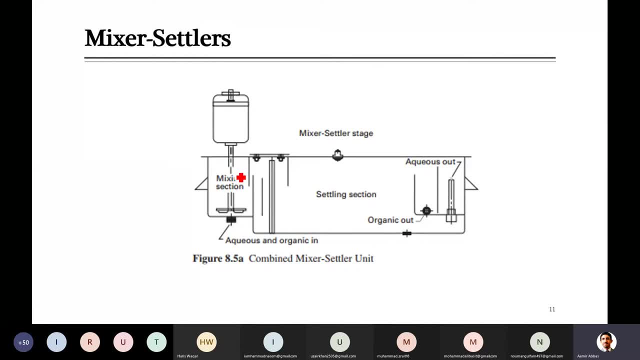 feed is introduced and solvent as well as the feed, and then you give them time to get settled. so overall, this again consists of two stages: separate stages, mixing within a separate stage and then there is a complete settling section. but they are just combined with each other. they are not working as a two separate. 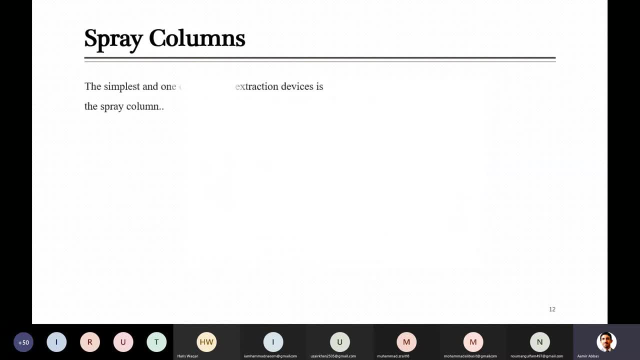 units, although inside one unit there will be two different stages. so the next common type of equipment which is used is the spray column. so from here actually we are going to talk about those equipment in which usually you don't have any kind of mechanical education. inside the first equipment which we- we we- have discussed like mixer settler, that is the 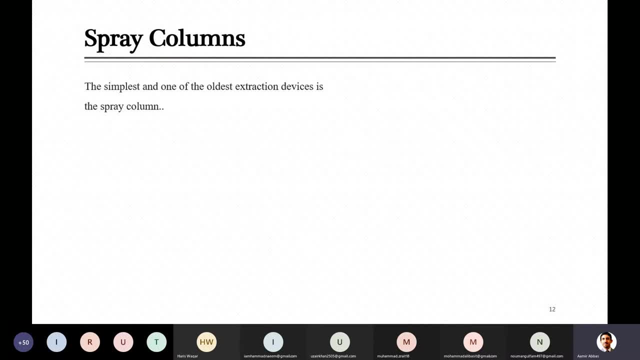 simplest device in which you can introduce mixing with the help of some mixing elements. but in the equipments which we are just starting there are three like spray column, then packed and tray, which we have to discuss today. so these do not involve any kind of mixing. so there will be 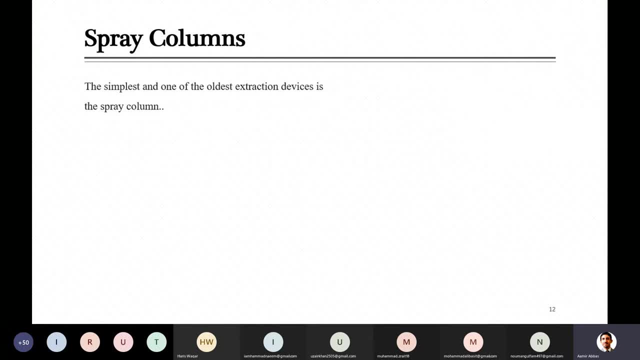 a spray column in which you will bring in contact the feed and the liquid solvent, so spray column. they are also the simplest and oldest extraction equipment. so in these this is the actually diagram which was shown earlier in the last. so this is for spray column, in which a spray, as you know already, 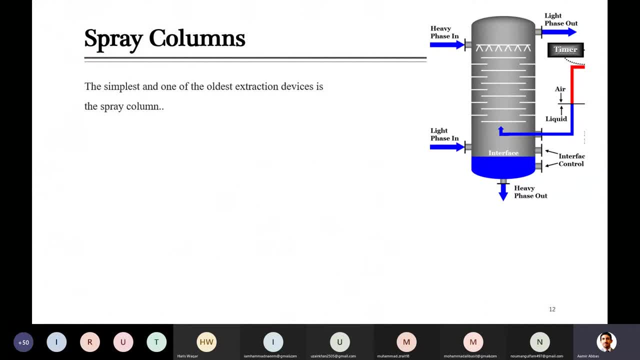 that spray column are simply those columns in which we just spray any liquid from the top. uh, already discussed related to the absorption. in those there was a liquid was spread from the top and gas was introduced from the bottom. but because here we have both in the form of the 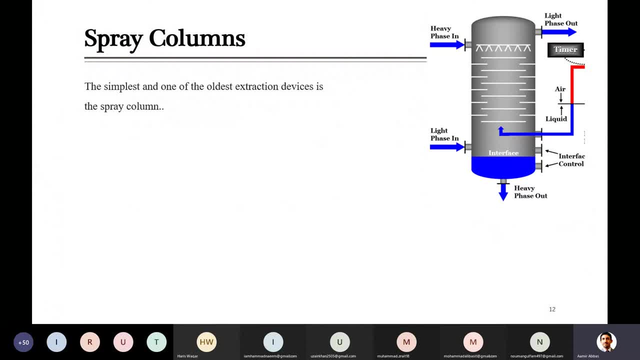 liquid. so one liquid will be introduced from the top, another liquid is just introduced from the bottom and they contact with each other. mostly they are just open, like there is nothing inside the vessel. uh, there are no, any prolactin or flakes or something, so the liquid will just. uh, heavy liquid is introduced from the top because, uh, it will definitely go down. 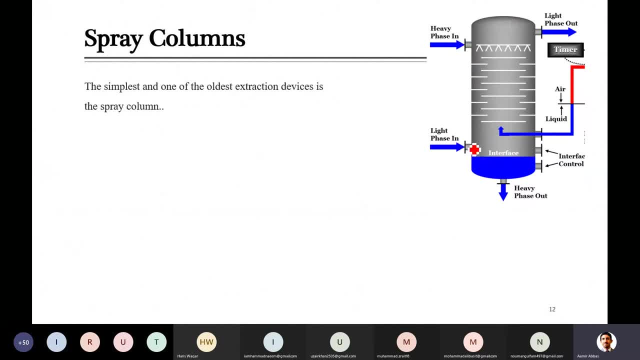 due to the gravity, as the lighter is just introduced so that it can just move when heavier is leaving, coming down, so it is just replaced and go to the top. so in the same equipment, here the like contact between the two feet and the solvent takes place, and then from the same equipment. 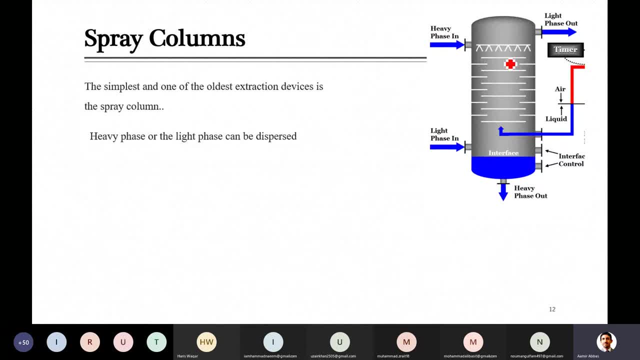 and refinate leaves at them. so, uh, this is, by the way, diagram from one of the uh main industry. so who are sorry manufacturers? so who manufactured these kind of devices? so maybe they have provided some extra details, but what you need is just, uh, you know the major structure of the equipment. it 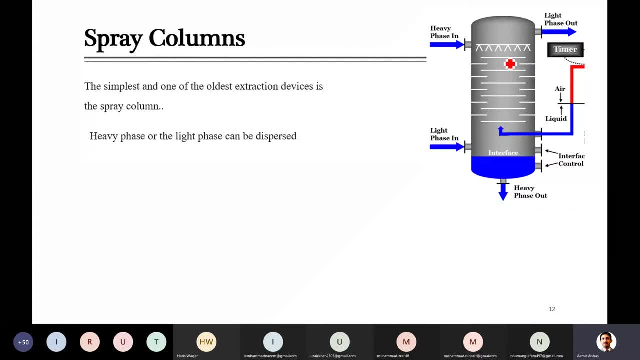 is also shown, i think, in your uh textbook. i have diagram here for you, so i will phase out the light phase. any of these can be dispersed. as i already told you that in this kind of equipment, uh, in which there is no mixing inside the equipment, there are no mixing element inside. 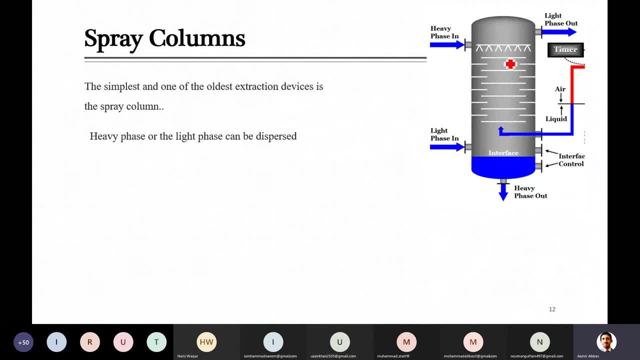 the equipment. so always we need to disperse one of the phase. disperse mean that should be discontinuous, that should be in the form of like droplets. actually the purpose is to increase the mass transfer. so other is like simply uh, so uh, here in these equipment either, you can just like. 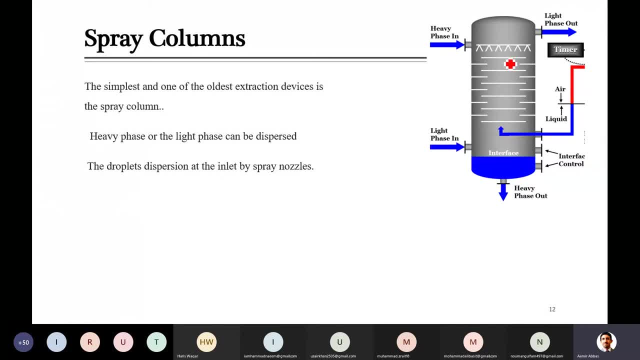 have a heavy phase or the light phase. any of these can be dispersed so that you can increase the contact. so, uh, droplet dispersion is done with the help of simple spray nozzle. so uh, in these kind of equipment, uh, there is one problem. just for a look, for example, heavier components are coming down and 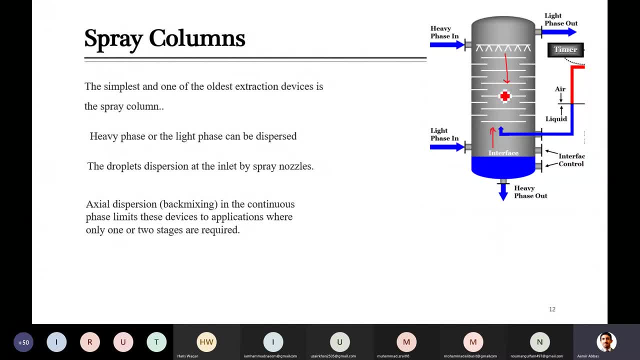 lighter are moving up and they are coming in contact with each other, so they will be technically mass transfer and okay if they are just moving in the vertical direction. they are moving in the vertical direction, it is okay, it is so fun to go with. but what happens in these equipment? because 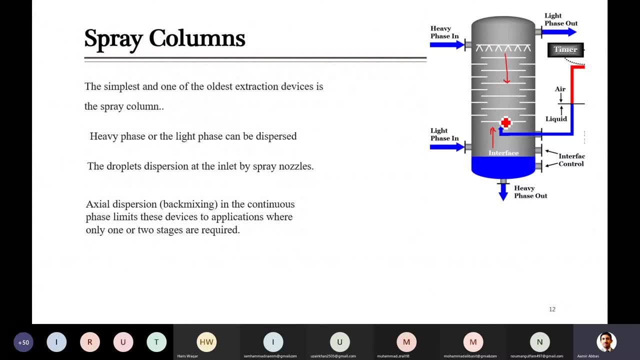 they are. we really don't have internal, there is nothing, there is simple vessel. so what happens? for example, any, any component or any molecule here from, uh this, instead of going to the top, it starts moving in this direction, axial direction. so when it will be moving in the axial direction? 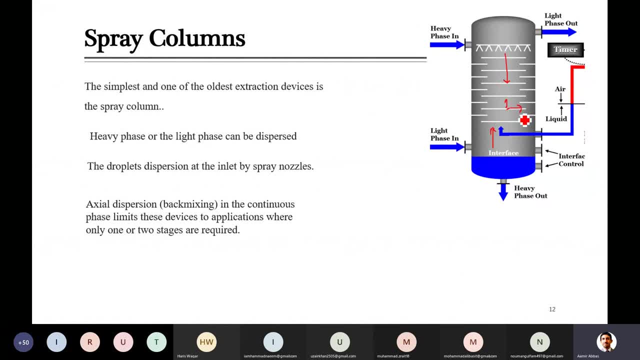 maybe if mass transfer it has already taken place, it can go back or it can reverse. so in these kind of equipment this is one problem which they generally call it back mixing. so whenever- uh, you know from multi-direction engineering also- back mixing takes place, so that leads to the problem, uh, that will reduce the efficiency of that equipment. so in 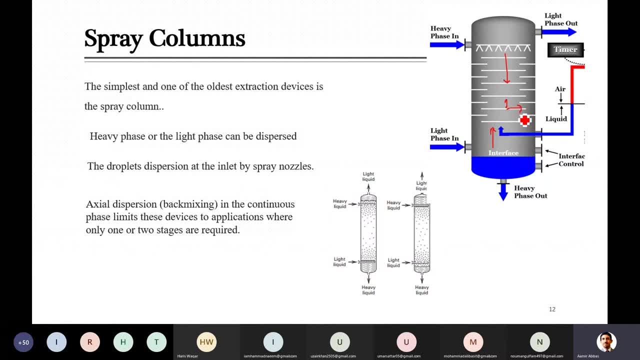 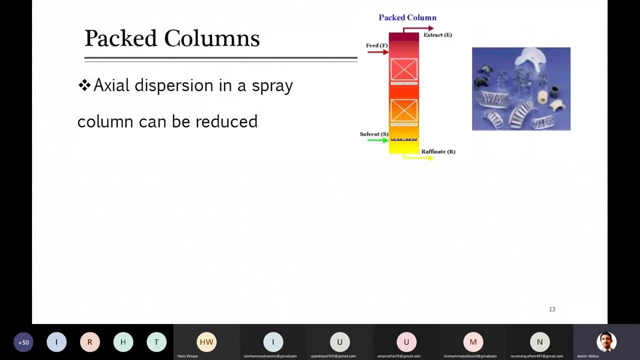 these equipment. the major problem is this one. so this is the simplest diagram related to these equipment. like you, are introducing something from the top, heavier one and lighter, from the bottom right, and the collar is the only important thing for us at the bottom. realize that this enroute. 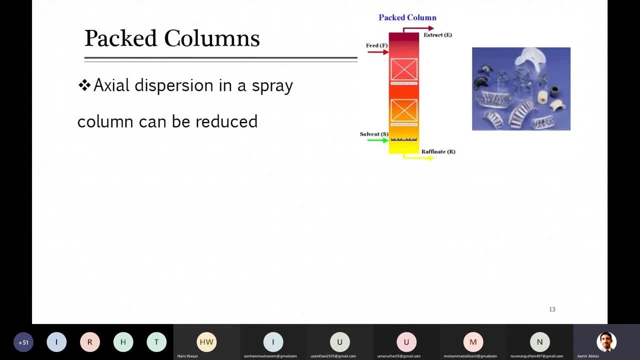 action director exercise. the other next equipment is the tech column. as i told you that in a spray column the problem is xvl dispersion, because in those equipment there is nothing inside the vessel, only liquids are. that can be somehow avoided if you just put some, uh, some packings inside the equipment. so 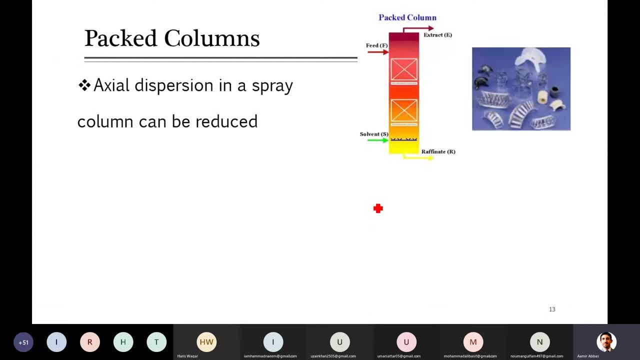 a pack column help you to reduce or inside these equipment, axial, like this person is reduced. the reason is like, when there are the packing, so at least there is some restriction for the flow of the liquid in, like very random. so, uh, here, when you are using the packing, as already, uh, you know. 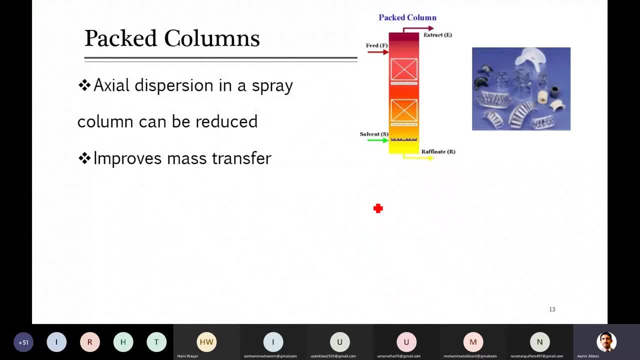 about the packing that when we introduce the packing they provide you more contact between the various fluid, like earlier it was liquid and gas in case of absorption, but here in the pet column, uh, when you are using it for liquid detection. so there will be definitely both of the liquid. 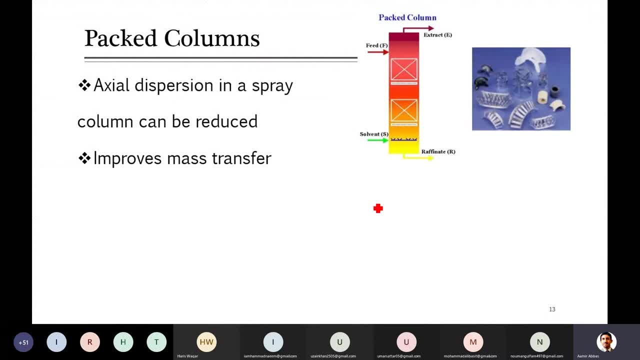 so inside these equipment already you know that one phase is continuous and other is dispersed. so their contact on the surface of like these different packings, so that is enhanced. or there is more, because when one fluid is flowing on the surface of like packing, so definitely that is more distributed as compared. 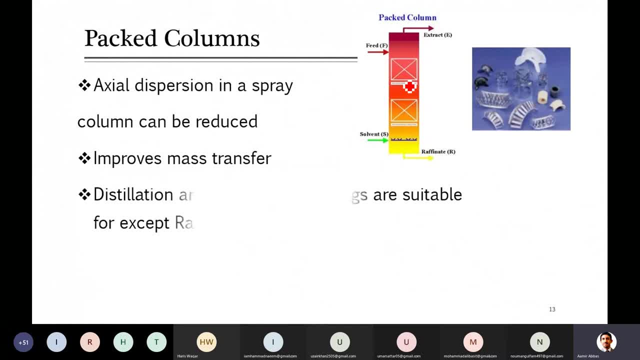 to if it was just passing through the column and the direction of gravity. so, uh like, distillation and absorption packing, uh, which you already know, there are number of different packings which were used for this kind of application, like for lle, except ration ring. so, uh, here there is a small 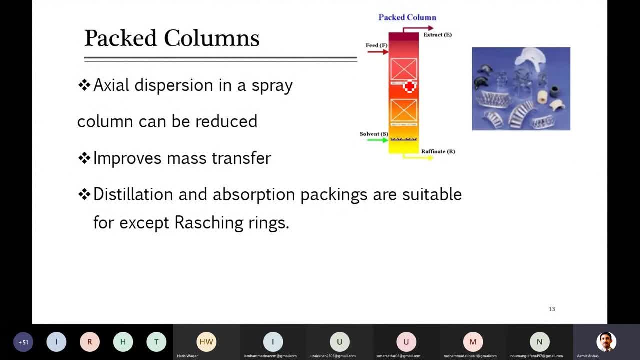 like assignment for you, or with this point you have to look. uh, for this you have to go back to the absorption packing in in the chapter of absorption we have already discussed, and look, uh, what ration ring is and uh, just think why it is not suitable for liquid. 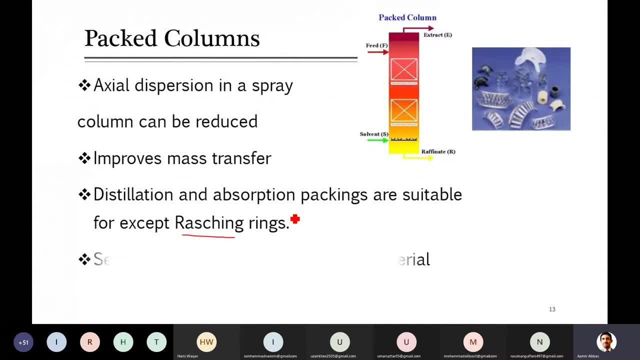 selection, and maybe i can ask you next time. so i just look for the reason. if you will study the structure of various packing, definitely you will come across the onset, that why it is not suitable or better selection. so, uh, here like selection of our importance of the packing material, uh, 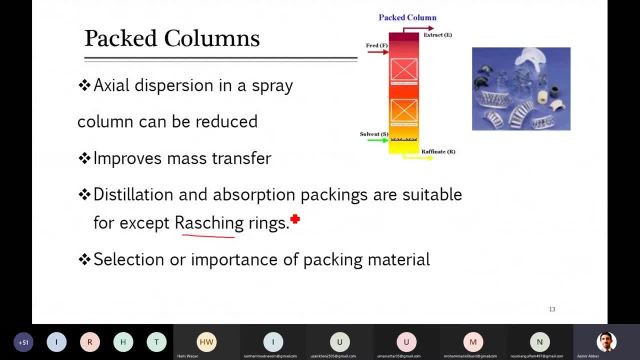 that should be said, that it can give like on the surface of that packing you can have a better liquid distribution, so so that more mass transfer can take place. so uh there. but the problem here in these kind of equipment, either spray column or pack column, so they are not, i mean like that- efficient. the reason 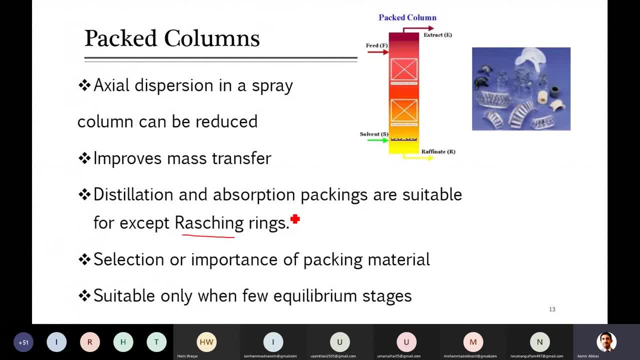 is like you are not like doing mixing inside the equipment, although packing help you to increase the mass transfer, but when there is not agitation or complete mixing, so that will like take more time for the two components to come in contact with each other and reach equilibrium, or the far. 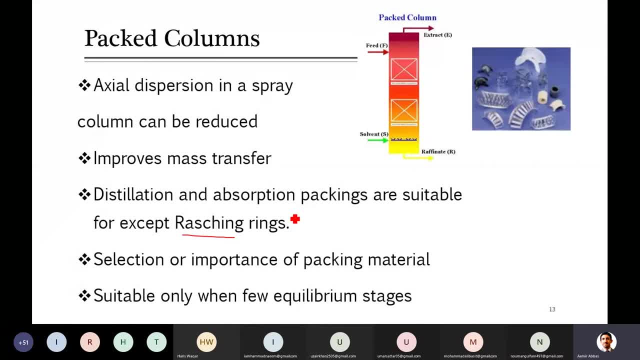 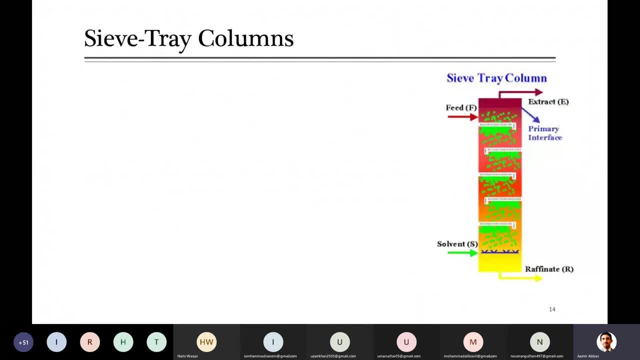 mass transfer. so due to this season, these equipment are just preferred if you need uh small scale separation and you just need two stages. but if vigorous uh like are heavy or higher separation is needed, then it is better to go for some other kind of equipment which will 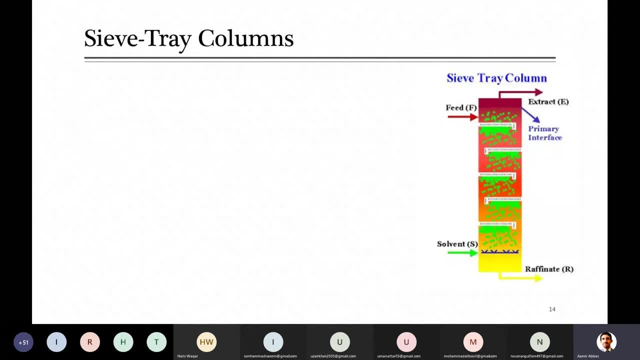 be discussed in the next lectures which are related to, like uh, mechanical education equipment. so, uh, then the third one here in this category is the sieve gray column, sieve tray. so uh, as this is gray column but the trays are only a c type. so in these kind of equipment, uh, sieve trays. 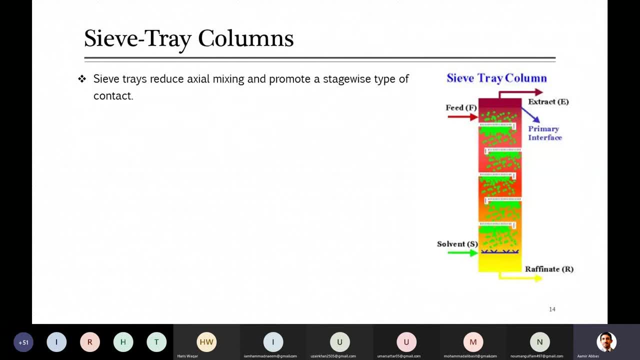 so they also reduce like actual mixing and uh, here statewide type of context take place. uh, in inside actually a separate column, back mixing is large, but uh, in the third one we also have a whole at one. but in case of these either back column or tray tower, that can be avoided. then in these equipment, 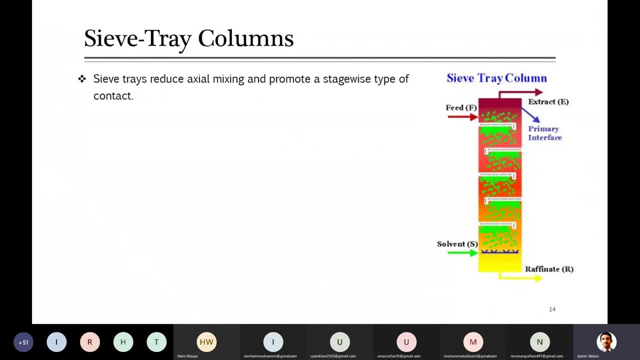 when we are avoiding that back mixing. definitely they help you to increase the efficiency. so in this equipment- again same- there is column. inside, trays or plates are given and i will just talk about this. the construction of these trays is a different as compared to the things which we know. 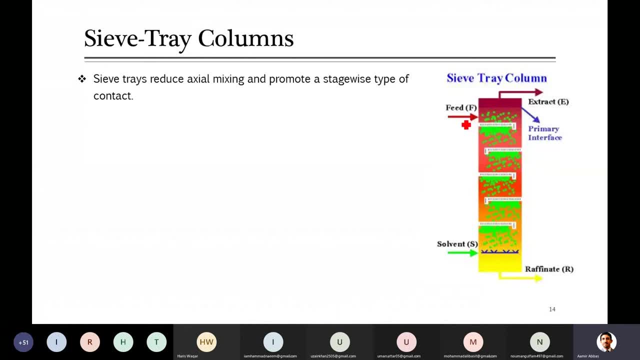 related to the distillation or absorption. so one one of the field or the solvent that is introduced from the top and other is introduced from the bottom. so, uh, it depends on the density difference. so definitely the heavier one will be introduced from the top and lighter one will be. 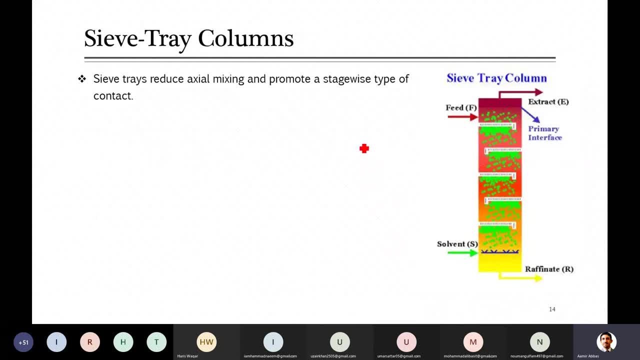 introduced on the bottom, so they start coming in contact with each other on the surface of, uh like trays, and then, uh, at the end they are just separated, leave from the and the bottom of the column. so dispersed space, uh like a here dispersed width, is something which 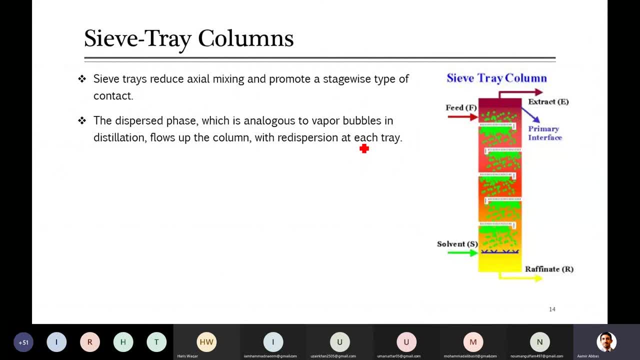 is like analogous to vapor bubble already. uh, we know that inside these spray column usually vapor guest go. that is mostly the dispersed space. so here, uh, one will be the discharge phase, which will be uh like related to the vapor bubble, and other one which is like continuous, that will be. 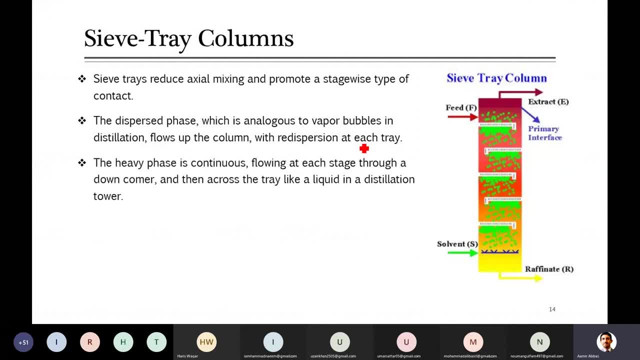 moving as a liquid um the surface of the tray. so heavy phase is continuous inside these equipment, flowing at each stage to a down comer and then across the tray and like the liquid, like heavy which is introduced from the top. that is continuous moving on the surface of tray then from the down comer. 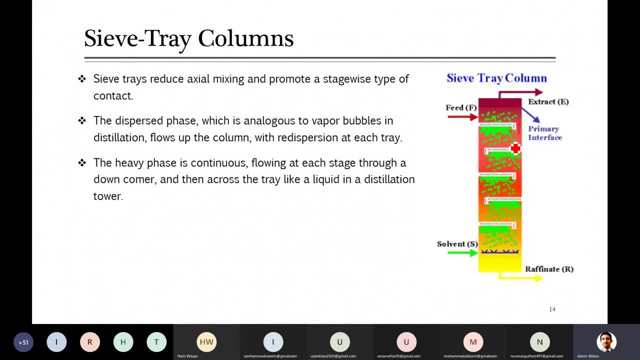 area like here, it comes to the next tray and then and so on, it keep on moving down towards the bottom of the column. so at the same time, the other one, which is lighter, which was introduced from the bottom and as heavy, will come down. definitely it will just move upward. so it will be moving upward. 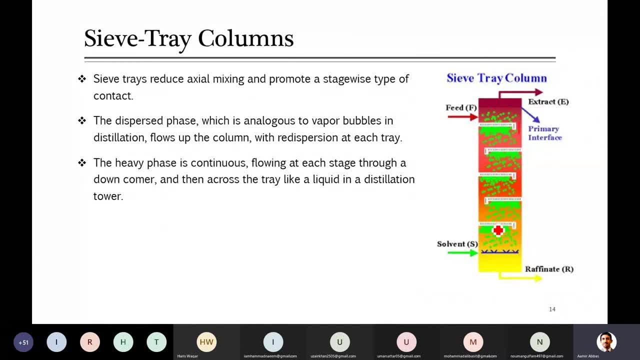 through the, i mean various holes inside the tray, because this is the seed tray, so they will be just moving towards the top through the hole. so, uh, column diameter in these case, because this is quite different from that- either distillation or absorption application, because here we are contacting 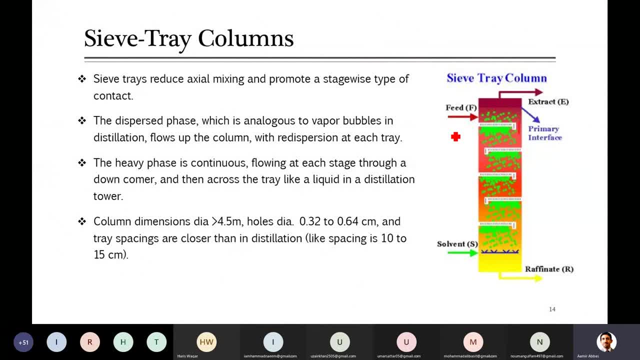 two: liquid, not vapor and liquid. so, uh, we need uh like that they should make better contact and the residence time should be more inside the column. their velocity should be low so that they can contact more as compared to the like when we use it, this type of column for the distillation or 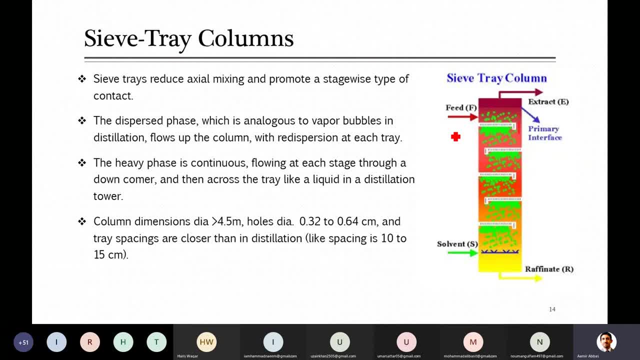 absorption. so, uh, like their dia is. usually the dia of these columns is greater than 4.5 meter and the reason is, when you are having a large column, velocity of the liquid inside the column will decrease, and when their velocity is decreased, so they will have more residence time inside the column and 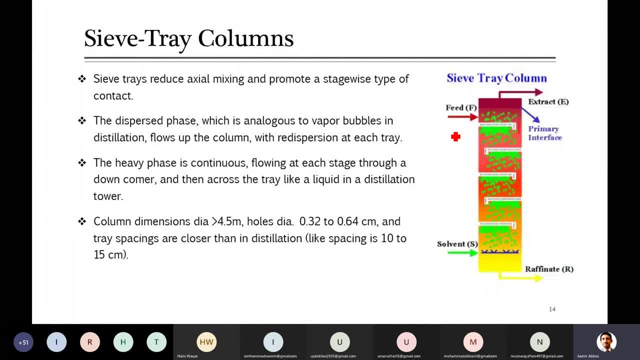 that will help you to get more mass transfer. so, uh, here the like whole diameter for the trays when we look at the seeds, so that is 0.32 to 0.6, so that is 0.32 to 0.6, so that is 0.32 to 0.6, 4 centimeter. and if you just go back somewhere to the 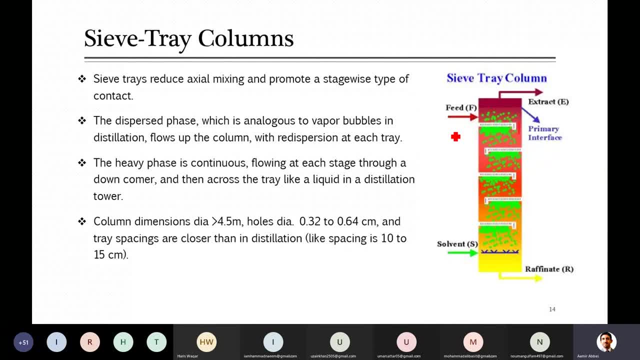 distillation or absorption and compare with those, these are the higher one as compared to those as well. the uh mean spacing between the holes is higher here. that is greater than usually more than one centimeter. so as well the tray spacing, but here that is closer than in the distillation column. so spacing here is just 10 to 15 centimeter and if we take it as a 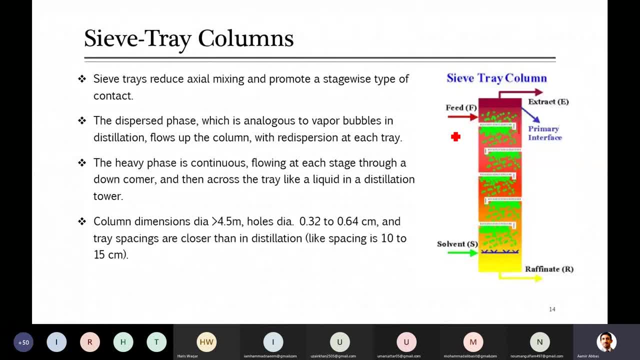 maximum like 15 centimeter. that is only half fit and you just remember from the absorption there. the spacing between the trays was around two feet, so 24 inch, or then more than this is usually recommended, and that the reason there was to avoid like or to provide the space for weapon. 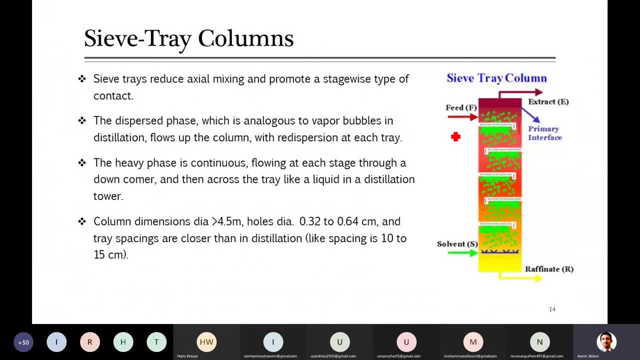 liquid disengagement as well if there is a foam formation, so there would be some space for like to avoid that problem. so inside these. but here because two liquids are moving, so we need more trays, more disturbance, so that when liquid are just coming in contact then they're like contact remains and then there is. 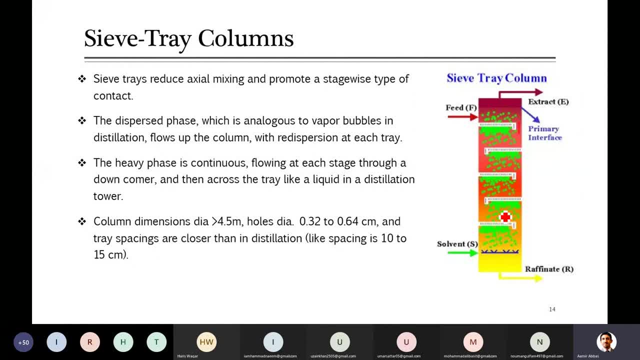 small spacing. after that again there is a tray. so here purpose of providing tray is to like provide the disturbance and in that case that can help you increase. so the another major difference in these column as compared to the previous one that is related to: uh, there are not outlet vias. so if you remember there were vias in case of 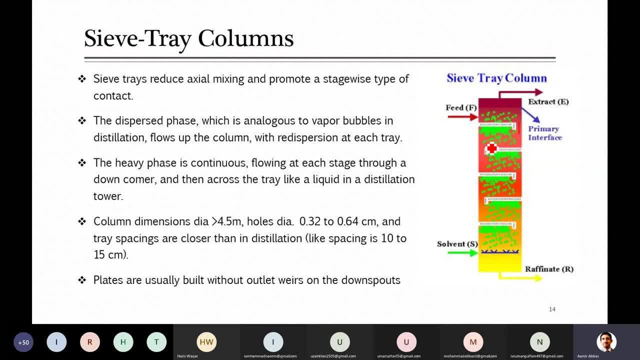 light. uh, when we talk about this, distribution are absorption. so here there are no weird. even in the diagram you can observe that they are not available. so any liquid coming, a heavier liquid coming on the surface of prey, they just move down towards the next plane and overall. 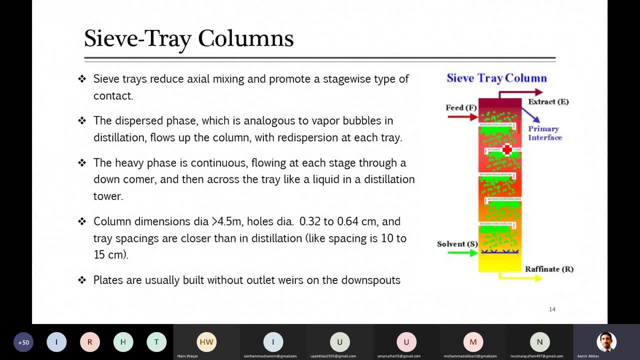 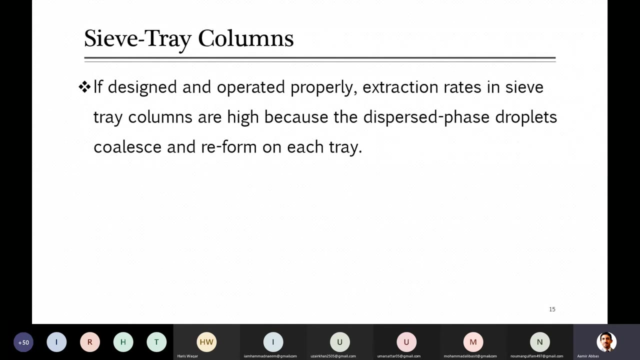 inside this column. when two liquids are conducted, there will be complete liquid inside the column, so they will be just contacting with each other and you don't need for these liquid to settle here for long and make contact with the other liquid. so if we just design them properly, like select, the spacing as well as other specification which 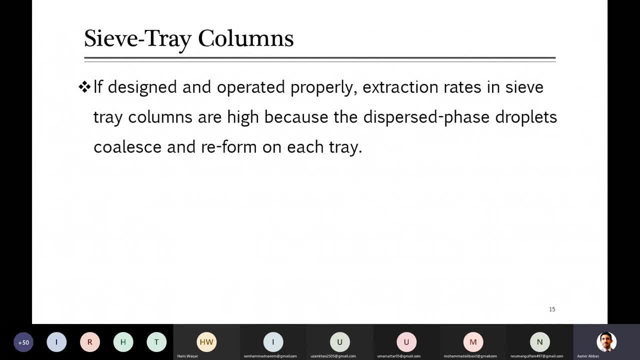 we have talked about. so extraction rate in these columns, see tray column- are higher. the reason is like dispersed phase droplets, well as, and then reform on each tray when they will just pass through the like droplets, sorry through the holes, if that is even continuous liquid when it passed. 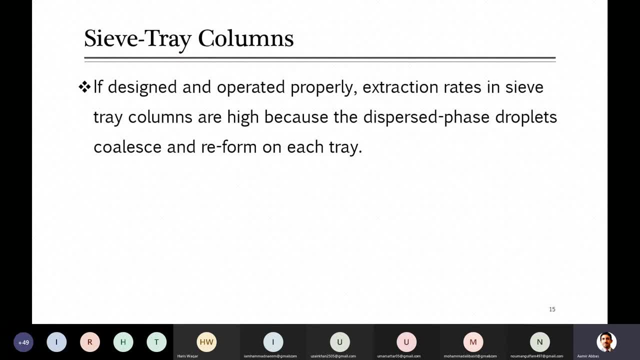 through the holes? definitely, it is just distributed in the form of droplets that is to break something large inside the small size polysense we call it. so then when they just pass through that tray, definitely they will again, they will make transfer, mass transfer with the feed and then, or maybe it is solvent so that 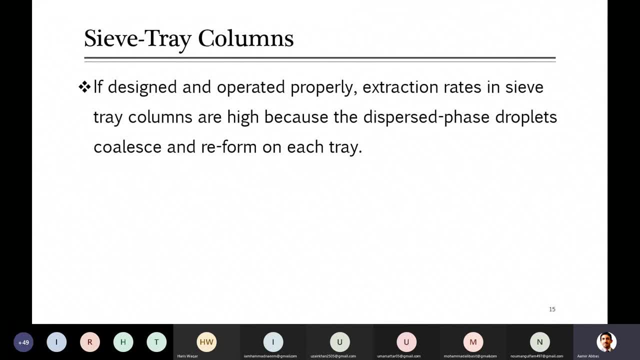 will make like mass transfer, and then they just join with each other, then another tray reads, and so on. this process keep on repeating. so due to this reason, we need less space and more number of trays here to increase this phenomena and to help in enhancing the mass transfer. so few tray. 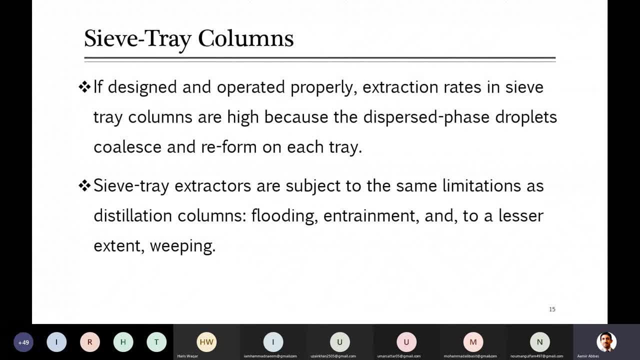 are subject to like same limitation as the distillation column. inside these even flooding entrainment can take place. suppose, if something is uh with like, for example, the lighter one which was introduced from the bottom, and if it is at uh like high flow rate as compared to the 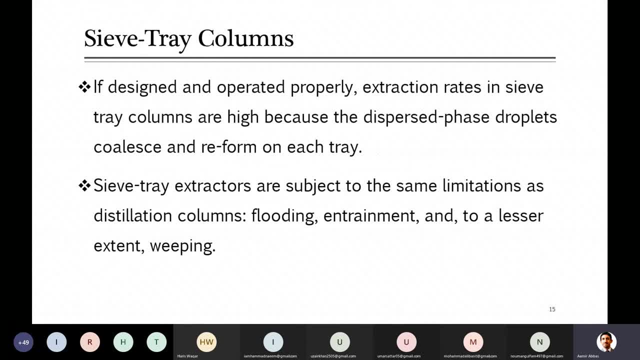 top liquid which was introduced from the top. so it can just push some of that liquid, as the vapor used to do in case of distillation or absorption. so, uh, even entrainment, entrainment was the case in which vapor were entrained inside the liquid. so if like, 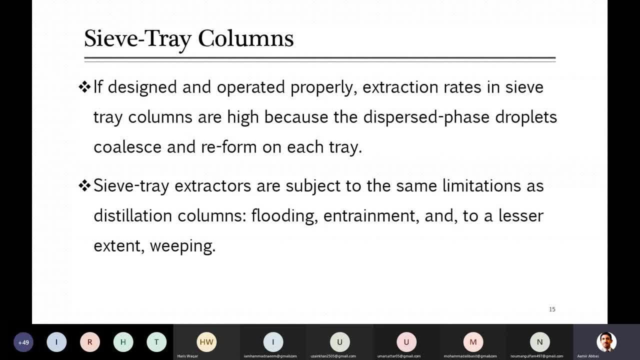 flow rate of heavier flow which was introduced from the top. if that is very high as compared to the one which is introduced from the bottom, so in that case that can push that liquid towards the bottom along with this when it is moving down. so these problems can also take place here. so in 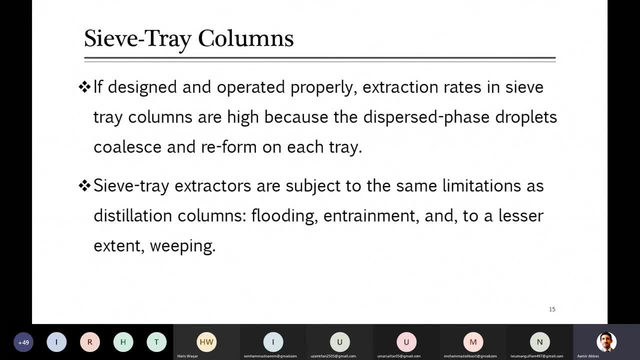 order to avoid them. definitely, we have to take care of the flow rates inside this column. so, but the problem, the phenomena of the sistole, is that. uh, so, depending on the flow rate, each of the three parameters can have a different flow rate, for example, that they have any room at the bottom.